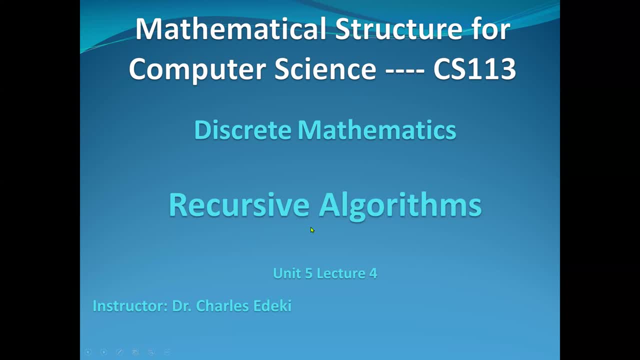 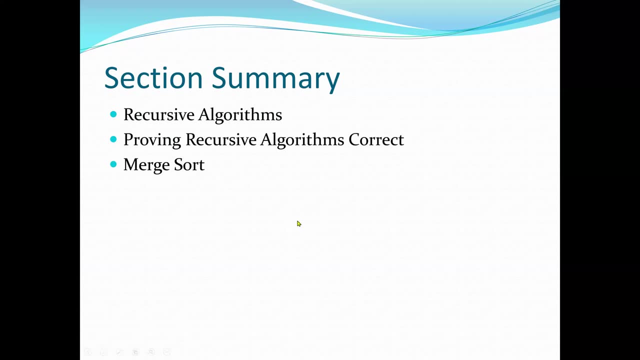 recursive definition functions. Our main objective in these lectures is to go through recursive logarithms which we have to use. the concept of a recursion or recursive functions, how it works. In our previous lectures we said recursive functions have two parts: the basis, 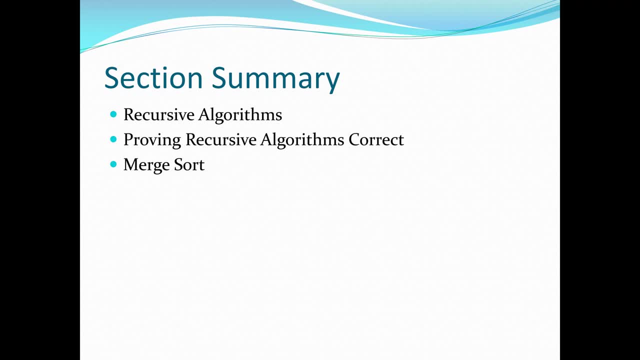 and the recursive part also The same thing. if we are going to write an algorithm using recursion, then we must have the basis step and also the recursively step. We'll see some few logarithms using recursion. Also, we are going to prove if a recursive 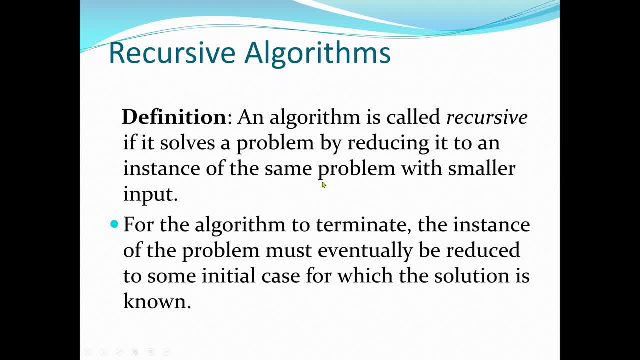 algorithm is correct. First we start with the definition. But first, what is an algorithm? We know an algorithm will be a step-by-step task that we normally do do to accomplish something, a function. An example would be: if I want to get ready to, 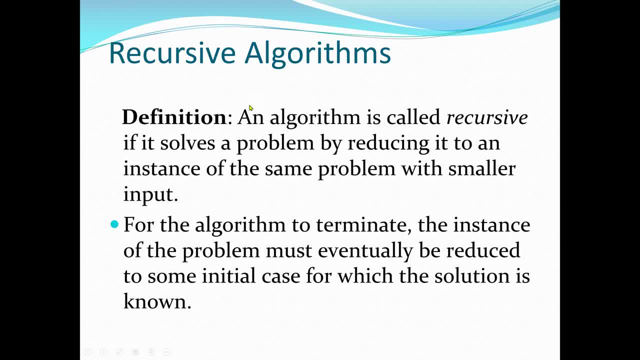 go to work, the first thing I need to do is to take a shower. Maybe when I wake up, maybe take a shower, clean myself up before I put on my clothes. So Garudim is step by step in very sequential order. Now, if I want to get ready to work and I put on my clothes, 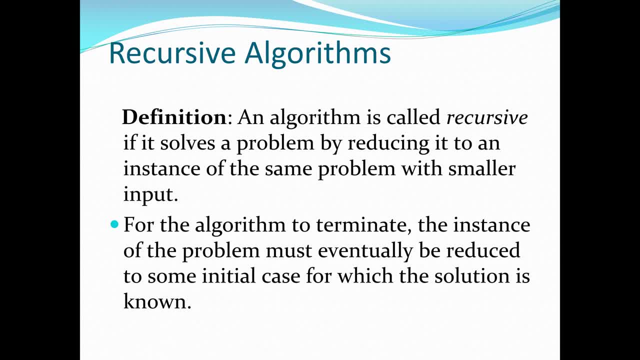 first before I take shower. well, the end result will not be good. I don't want to go to work with a wet clothes on, or maybe there'll be soap everywhere. So that's the concept of our Garudim. Garudim is solving a problem or performing any task by following some step. 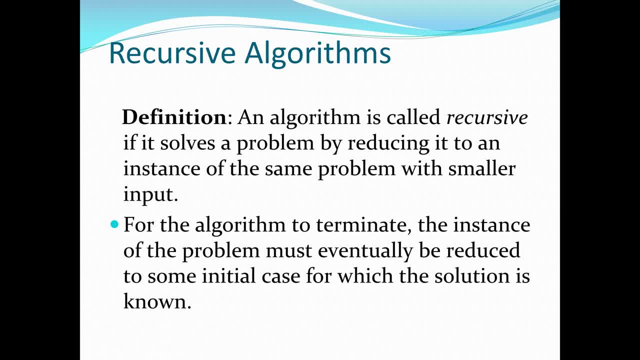 in sequential order. First thing must be done first. second thing must be done second, and they have to be in a duration of time. There must be a time period to finish the task. So that will lead us to recursive for Garudim. So recursive for Garudim again is the same as our Garudim, but this 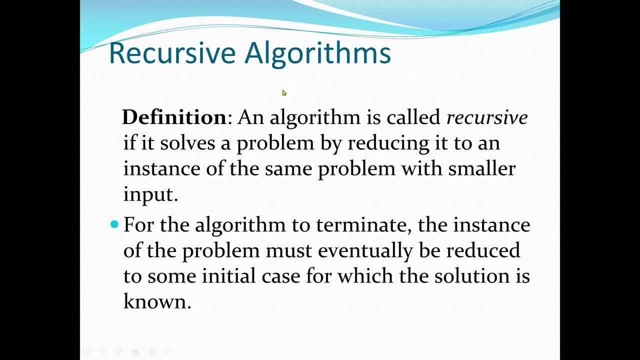 time we are going to use the recursive method to solve the problem. So the recursive method is the definition we have here, And a Garudim is called recursive if it solves the problem by reducing it to an instance of the same problem with smaller input. So what we are trying to say is a recursive for. 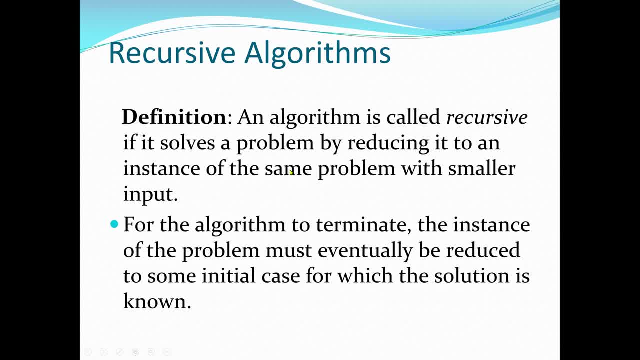 Garudim is a Garudim that normally reduce itself. So if I write a recursive function to solve the problem, the function must call itself by reducing up to the smaller input, And the smaller input normally will represent the basis step. Again, we went through recursion. 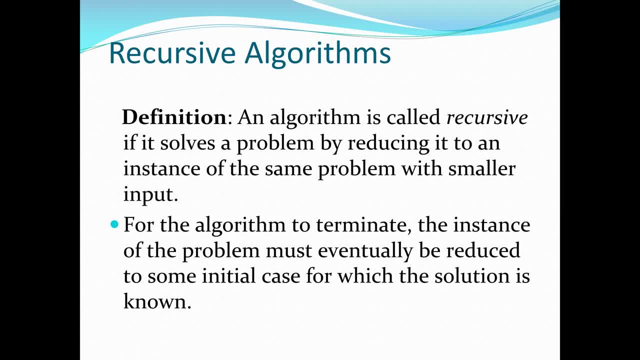 Recursion has two parts. We have the basis step and we have the recursive step. So normally if I'm going to find a factor of a number, the basis step will be: a factor of zero is one or a factor of one is one. That's the smallest input, zero or one. The reason I'm 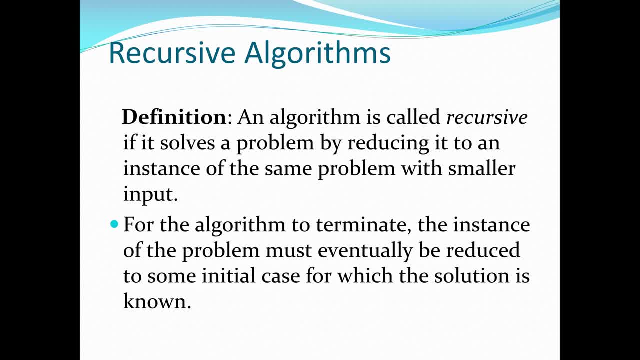 saying zero or one, because a factor of zero or one, the answer is the same: It's one, But we can choose only one. Let's say a factor of zero. Now, if my question said I should find a factor of five, then in my recursive step I will start from five times The function. 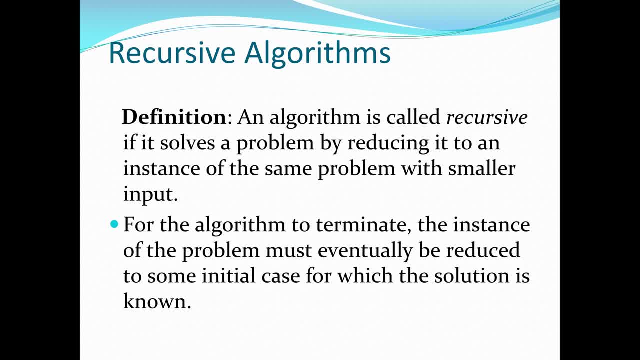 will call itself by reducing one, So it will be five times four. It will call itself by reducing one. three Call itself by reducing three. Call itself by reducing one. two Call itself by reducing one. Now, any time we reduce by. 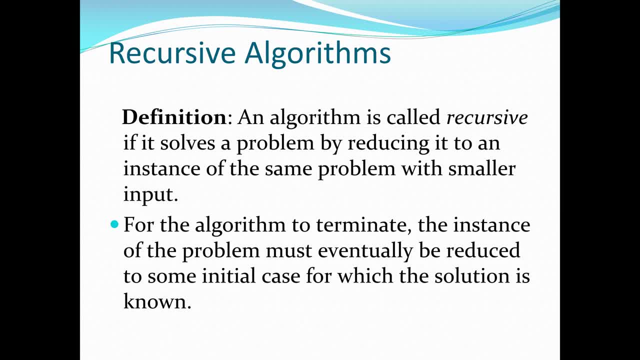 one. we have to check with the base condition if the condition is true or false. Now, if the condition is true that our smallest unit is one, then we stop, Then we give our final result that we have from the reoccurrence in of five. 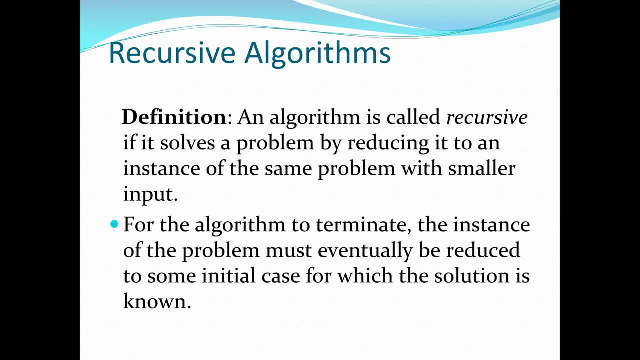 Then we give our final result that we have from the function calling the function over. If it's false, then we keep calling out. That means we have reached the smaller input here. So again, an algorithm is called recursive if it solves a problem by reducing it to an. 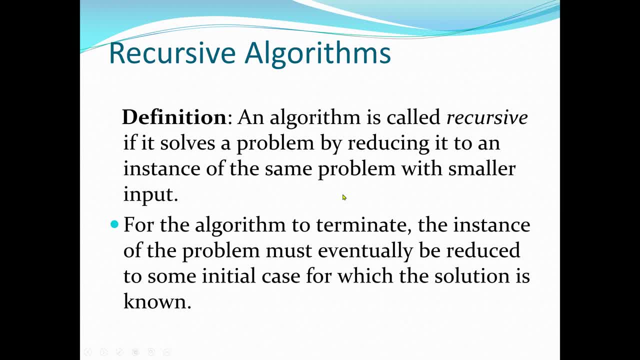 instance of the same problem, So a factor of a number. you can see that we have five times, four times, three times. So it's like repeating the same thing. Reduce it by one, multiply, Reduce it by one. But if it's a problem you can reduce it by one, But if 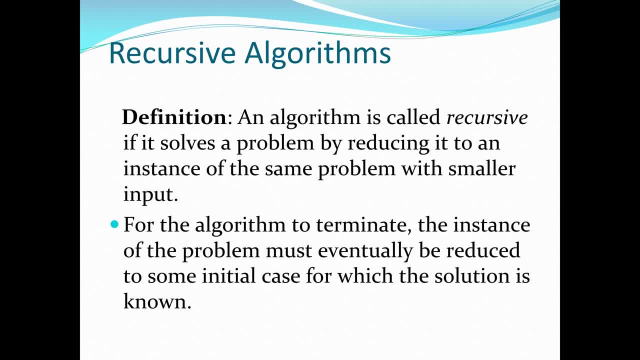 I want to find a product of a value that it will be 100 times 92 times 87 times three times four. again, we can see that it's not the same any time. it's reducing is we are not doing the same task because the difference, the intervals, are not the same from 100 to 97 to 20, back to five and six. 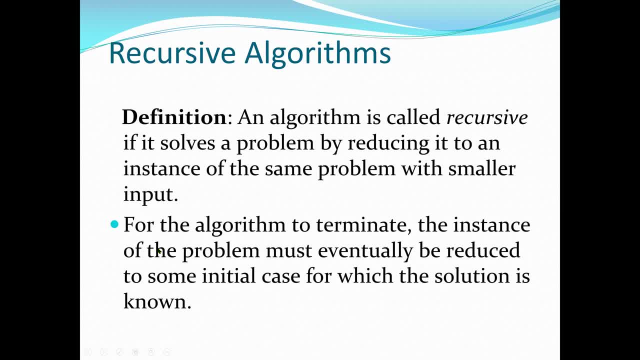 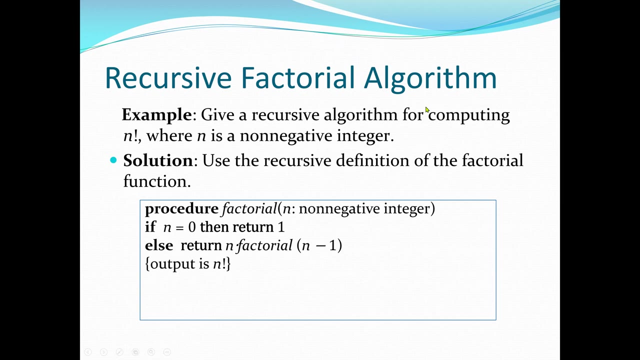 and we can't use recursion. so for the algorithm to terminate, as we said earlier, the instance of the program must eventually be reduced to some initial case for which the solution is known, which is the basis case. so example is given here: recursive factorial algorithm. so give the recursive algorithm for computing n factorial. 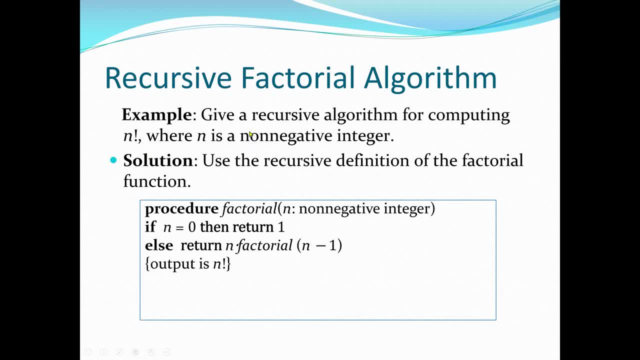 now in computer science we have something called looping or interactive. now i know a factor of a number means i will multiply the number by itself, by multiply the number to the next number, by reducing by one all the way to one. so, for example, if i'm looking for a factor of three, 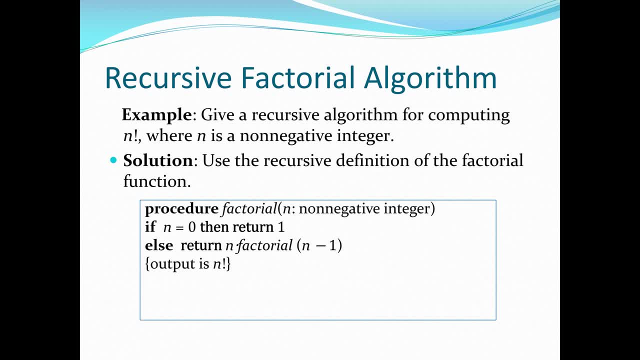 is three times two times one, or i can say one times two times three. this means i can use a loop to find a factor of a number. but when i have a loop, let's say i'm looking for a factor of 10, i'll say, okay, my loop will start from one and also it shouldn't go more. 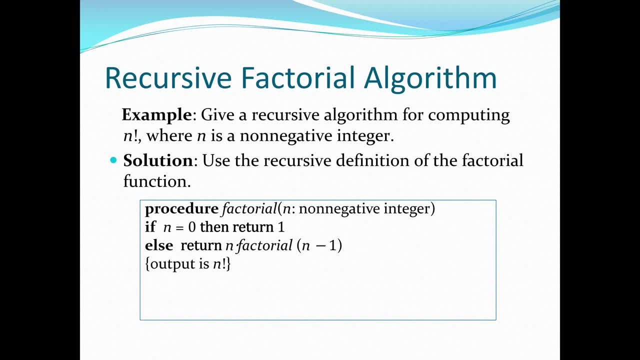 than 10. we are going to start from beginning, not more than 10. then we increment by one. so now my product. i will say: the counter equal today, the counter times. whatever we start, we start with one. so first we initialize the variable factorial as one, so one times the first value. then we increment the counter times the next. 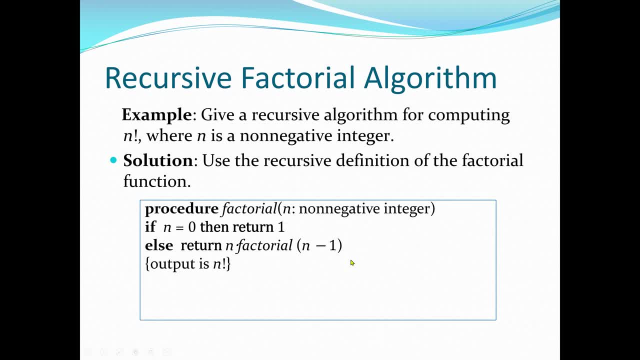 value increment. the counter times the next value. so at the end we're going to get one time. let's say, if it's factor of 10, then we get one times two times three times, four times five or the way to 10.. here i'm using a loop. let's say for loop. initialize my counter. i will start from one. 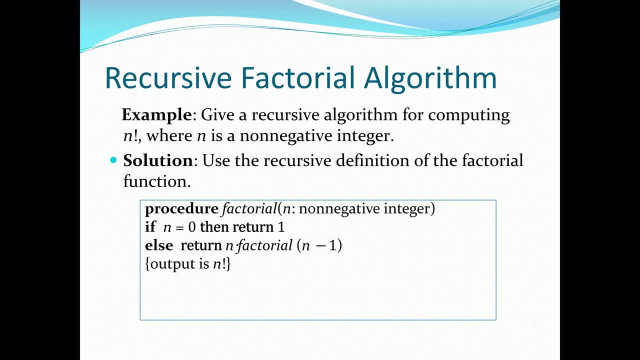 and the condition will be: this loop shouldn't go more than 10, so it should be less than or equal to 10 and we increment the counter. let's say the counter name is i, so i say i equal to i plus one. then inside i have a variable where i will store my factorial results. let's say we call the variable. 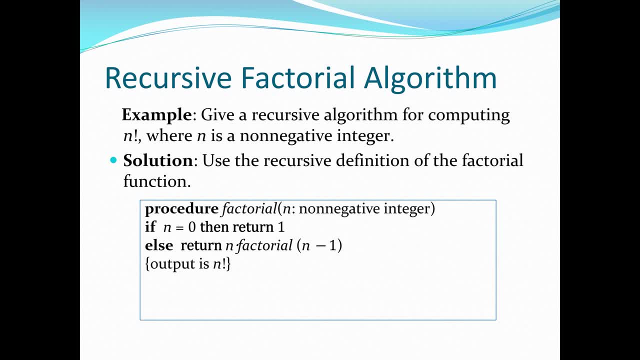 determined, so i can say: fact equal to fact times i, and i'll initialize the fact one, the beginning, because one times any values is the same value. so when i start with one, one times one is one, then we go to two, one times two is two, then we go to three, two times three. 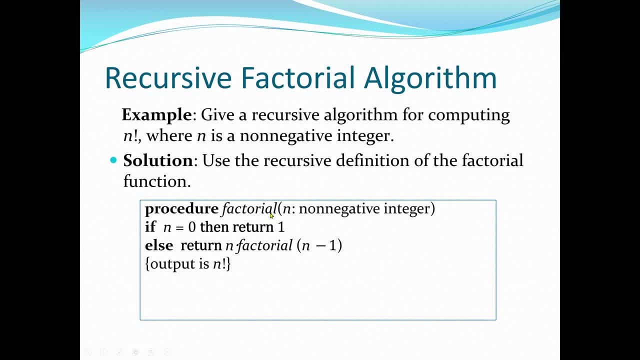 six. our result now is six. we go to four, six and four is twenty-four. our result now is twenty-four. when we move to five, it's 120, then we keep going. That's the way we solve a recursion problem using a loop. This is how we solve a factorial problem using a loop. Excuse me a factorial problem using. 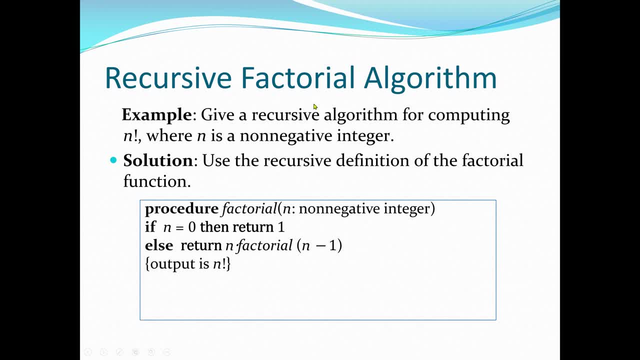 a loop Now to solve a factorial problem using recursion. we need two things. We say we need a base and a recursive. When we look at the algorithm here, we can see that here we are saying that if our input is zero, we'll return one, which means, if the factorial of 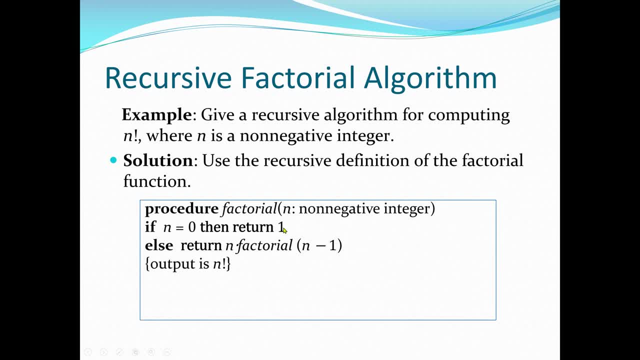 zero, the answer should be one. This would be our base case. If n equal to zero, return one. Else return n times factorial minus one. If it's a factorial of five, I would say five times four. The result I get, we check, We reduce by one, It's three equal. 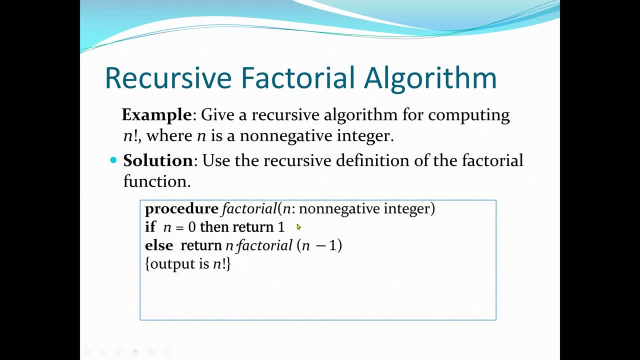 to: We've reached zero yet. No, We go to three, We go to two, We go to one, Then we go to zero. Zero, then we stop Zero. give us one. Whatever answer we get for the fact times, the answer we get before we reach one, we will return the answer to the function Here. 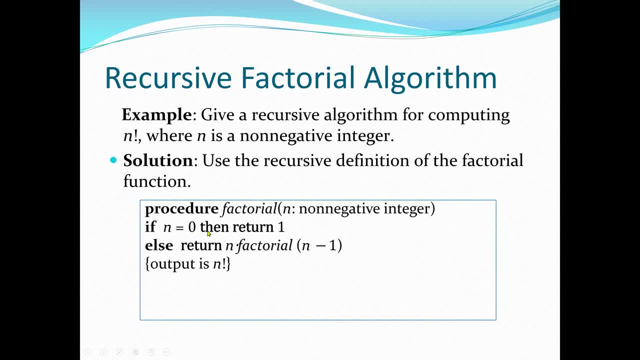 we have two. I'll use the term case. This would be my basis case. There's the smallest unit that will stop the recursion. Then this is my recursive rate. The formula will be n times factorial. The function is calling itself Again, the. 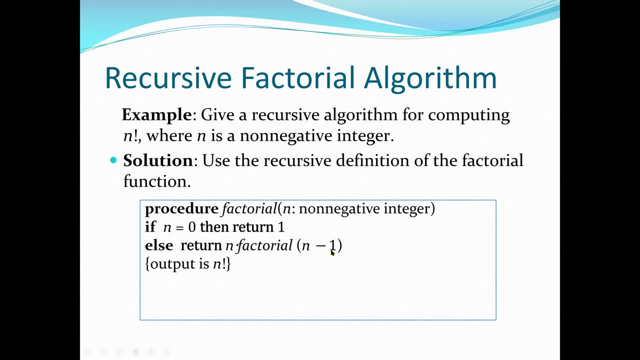 function in this factorial is calling itself: Reduce it by one If it's five, four, Next time it will be three, two. until this condition is true, If I reach n equal to zero, I will stop because I can't do anything. I'll return one. 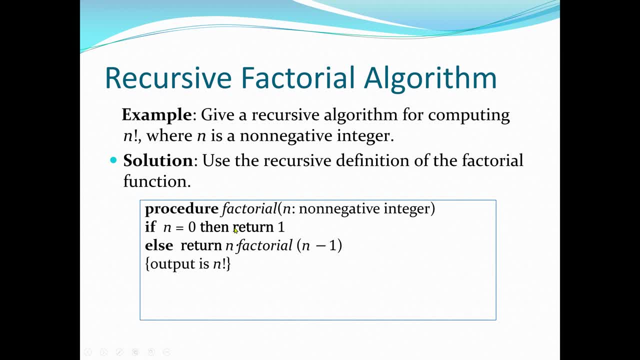 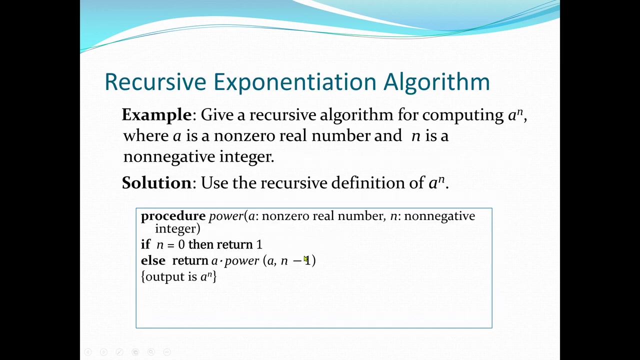 because that is the condition for the basis step. So again, this is the whole concept of recursive, using recursion for factorial algorithm. But what we want to know here is that in recursion we have two cases: the basis and also the interactive or, in this case, the recursive. So we have another example of recursive exponential. 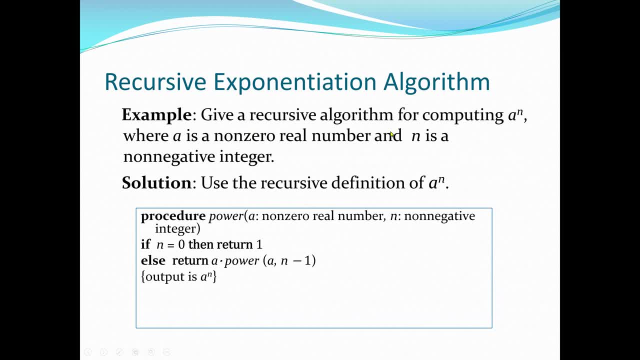 algorithm. So give a recursive algorithm for computing a to the power n, where a is a non-zero, zero number and n is a non-negative integer. Now here, a to the power n means a times, a times, a n times. But we are using recursion here. So first of all, I know that if I raise n, if n is a zero, 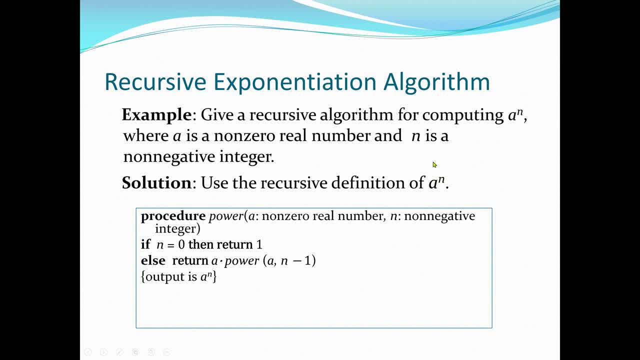 any value raised to the power zero is one, And that is the lowest unit n will reach. We don't need negative, So our basis case would be when n equal to zero will return one. Otherwise we are going to return the value times a to the power n minus one. 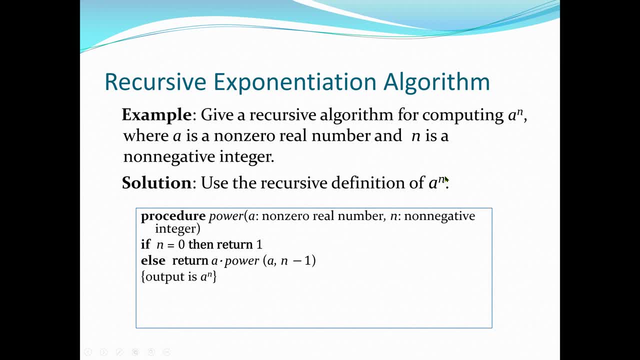 Since we take a out the n, if it's four it will be three. Next time we take one out, it will be two. Next time we reach zero, then we stop because zero is the condition for our basis step. So that's why recursive section we can see they say return a times the power. 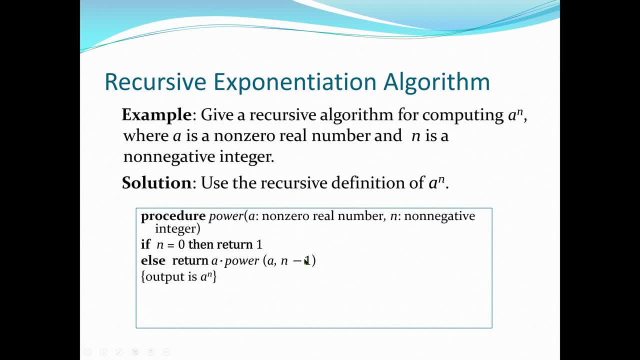 raise the power a by this time n minus one, because we take one a out, So it will be n minus one. So next time we get the answer, Next time it will be n minus one again, which is like n minus two, three. We go on to n reach zero. 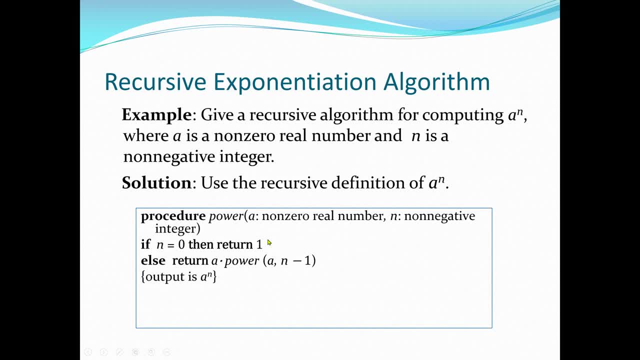 When we reach zero, the condition here will be true. Then we return the result, So the output will be a to the power n. So again, we know this concept already in arithmetic. but the whole thing we are learning here is how to design recursive. 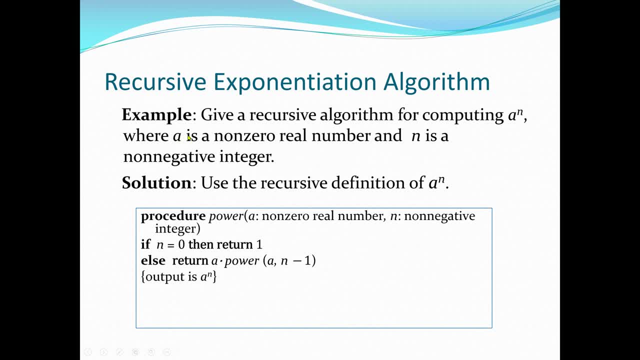 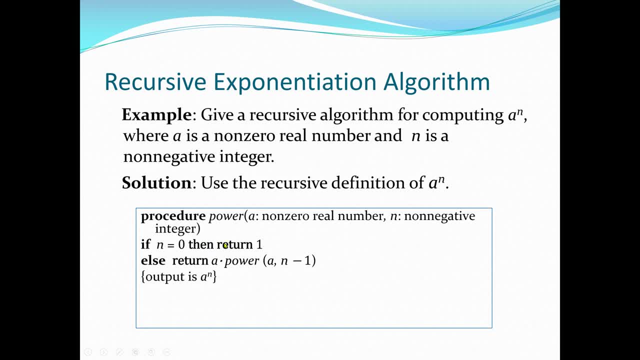 the recursion. if the condition is true, And always the base case will be the smallest input we can get. We can go. So here n should be zero. We don't want no negative positive values, so n will go up to 0. Any value raised to the power 0 is 1, so we say when n equals. 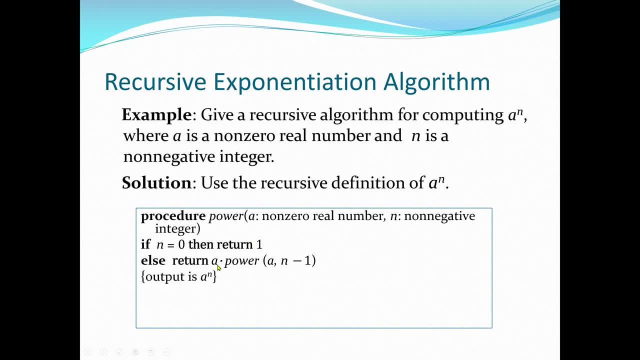 to 0,, we return 1.. Otherwise we return the value times the value raised to that power minus 1, because we take one value out already. So the power a n minus 1 will call itself until n minus 1 reaches 0.. Until n reaches 0,, then that will meet this condition. then 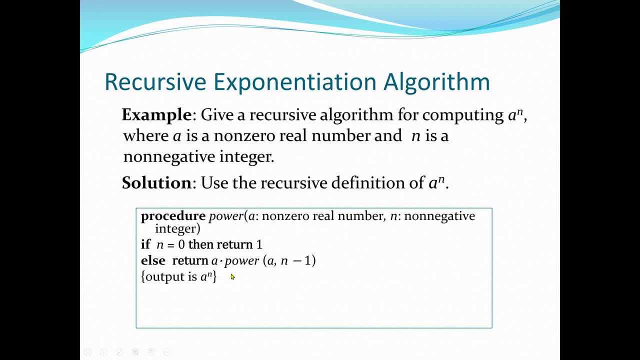 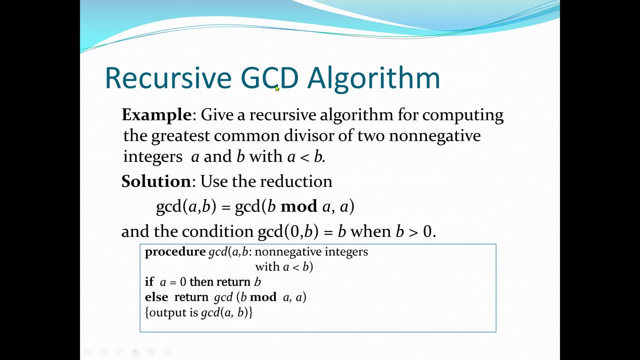 we stop and return the result. Another algorithm is greatest common divisor. What we mean by greatest common divisor algorithm? we find this a lot in fractions. Two values are given, maybe 2 and 4.. We can say: what is the GCD? GCD will be a number that is divisible. 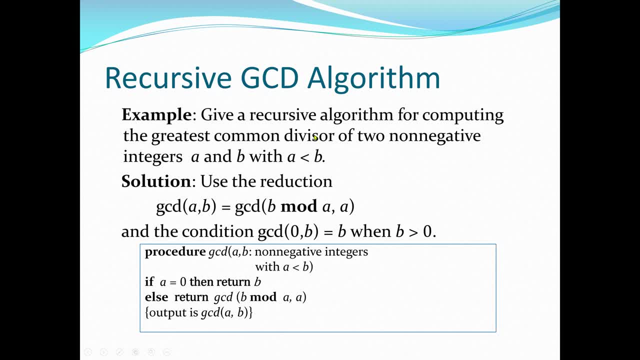 by both numbers. So if I have 2, 4, the GCD will be 4, because 2 can go into 4 and remain at 0. 4 can go into 4 and remain at 0. So here we have examples saying that give a recursive algorithm for. 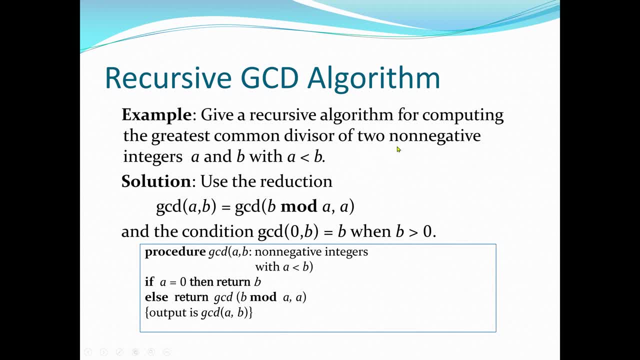 computing the greatest common divisor of two non-negative integers, a and b. But here we make sure that a is less than b. So for example, I have 2 and 4, not 4 and 2. So use the reduction GCD. a and b is the. 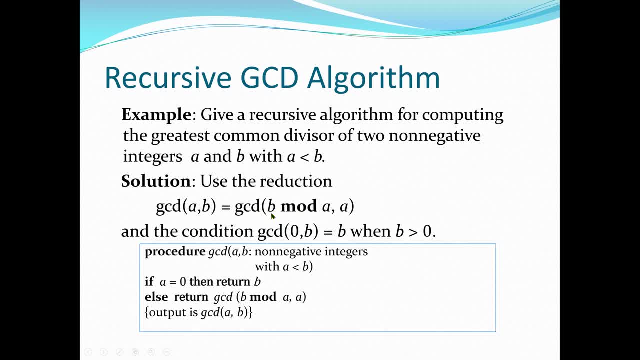 same. Same as saying GCD b mod a. Remember b is greater than a, So b modless a, and then the a variable And the condition GCD is 0, and then b will equal to b when b greater than 0.. 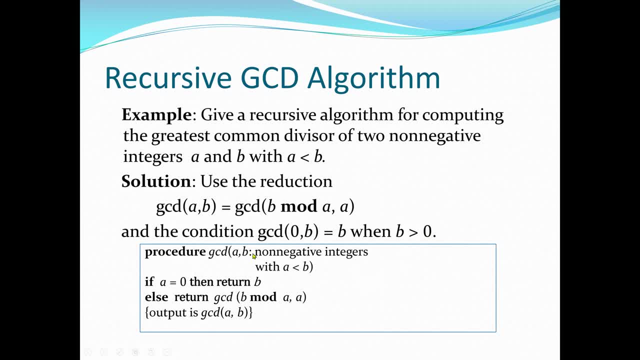 So maybe this should make us get the step. well, This means the lowest value for A always should be zero. If A is zero, what will happen? B will be the answer. For example, if I'm looking for GCD of six and 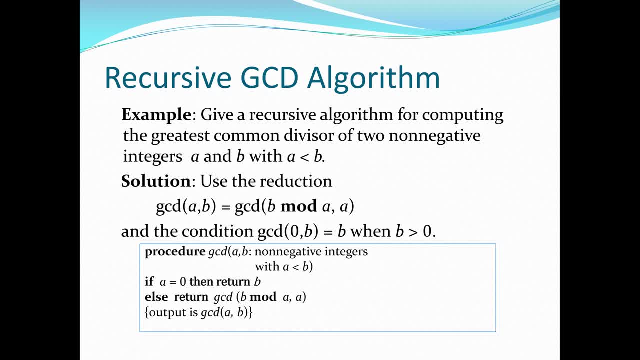 zero, the answer is six. Or one and zero, the answer is one. That's the basic step. When A equal to zero return B, As we return GCD B, mod A, remember the condition we have: A should be lesser than B. Actually, I should say two, four or zero, six or zero 10.. 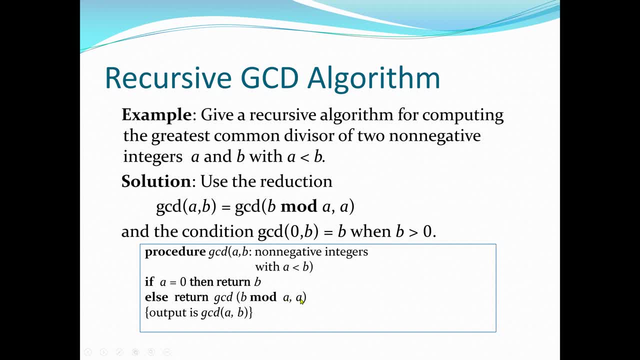 We say B mod A and A, The function have to call itself during this operation until A becomes zero. When A is zero, we return B. Then the final result will be the output of GCD A and B. Again, the whole concept here is using recursion. 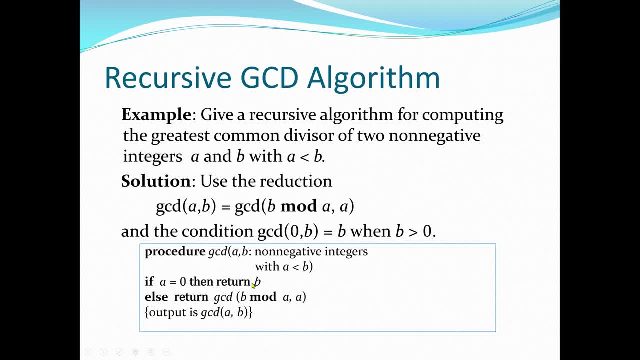 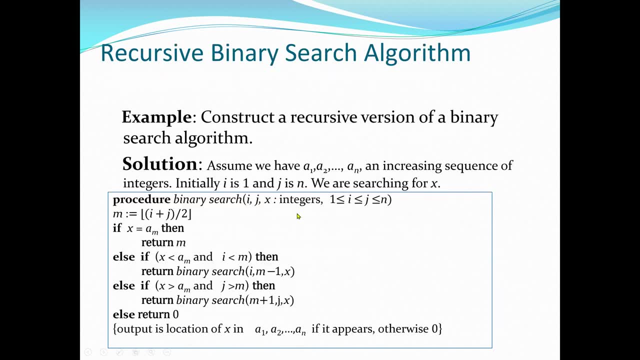 method. We have our basis case. Then we have our recur-city statement or case. Also we have the recursive binary search algorithm. Normally in computer science we have two common searching algorithms. One is linear search. Linear search means I have items in a list, Let's say we have A1, A2, up to A, and I want to search a specific. 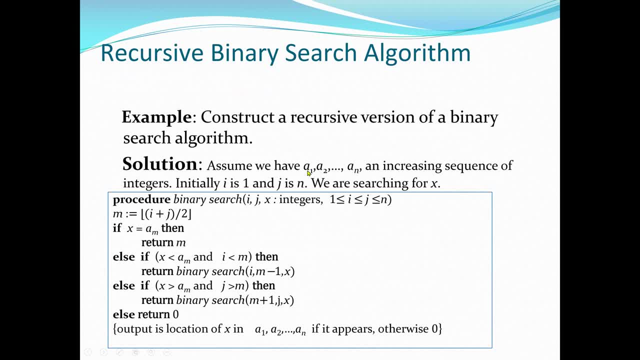 value. Linear search means I will start from A1 all the way to A. For example, if I start from A1 and the item I'm looking for was A1, I will stop. I'll return what I'm looking at, the position Now. if I'm looking for A3, I will compare A3 with A1. It's not it A3. 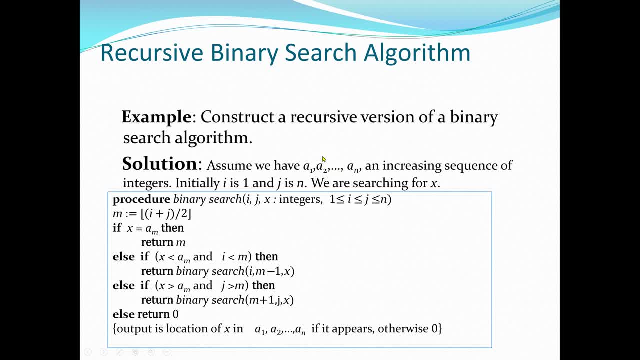 with A2, is not it A3, okay, we got the A3. Then we return A3. We stop searching. The worst case scenario It's when we don't have the item, or the item we are searching is at the end of the list. 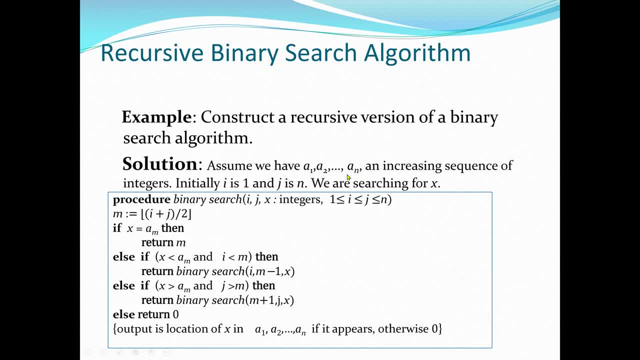 Then we have to do a lot of comparison, almost to the end. Linear search is good for small lists of items, but binary search is good for large lists of items, Because with binary search first we have to make sure the items are sorted. When the items are sorted we 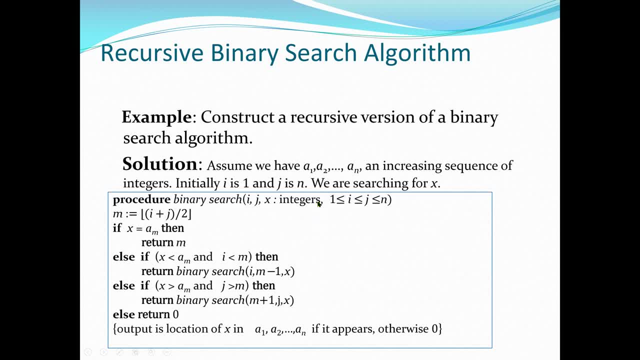 will look for the item. No, not the item. We need the item of value. So when we look for the item, we've sorted, if we make sense, if we do some arithmetical operation, we'll get the middle value. Then 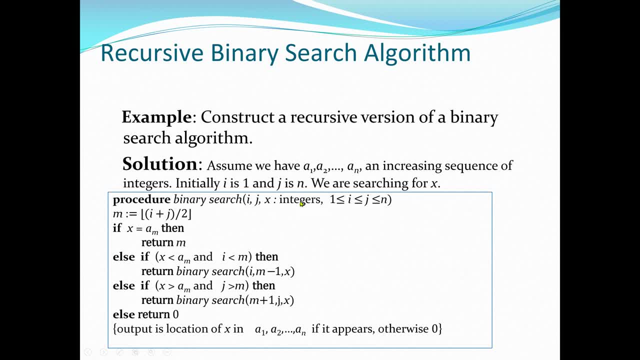 when we get the middle value, we will compare with the right or the left of the items between the middle, the item to the left of the middle, the item to the right. Whatever is true we go to. For example, if the middle item is less than the search key, then we'll go to the left. 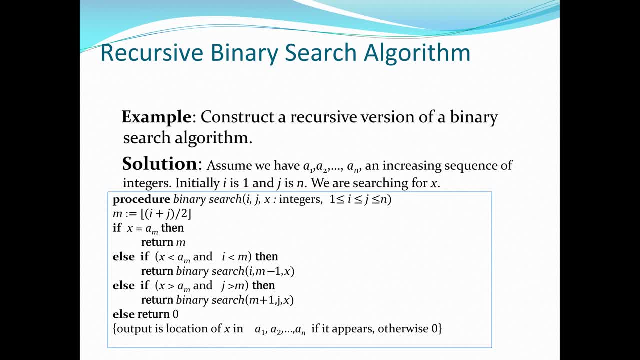 Middle value or the search key is greater than. sorry, if the search key I'm looking for is less than the middle value, then we'll go to the left side. Now, if the search key I'm looking for is greater than the middle value, that means after the middle value, the attempts to the right of the middle value are greater than this. 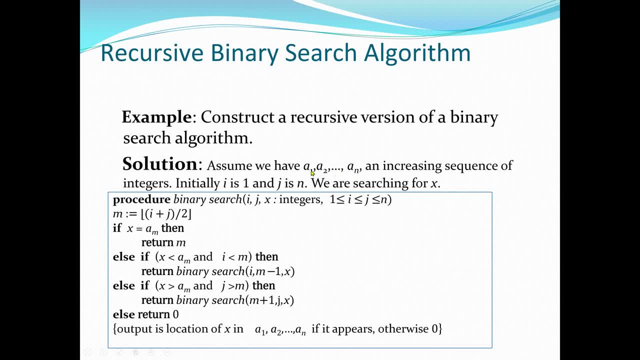 So we look for the right. So this means in our first searching, when we get a middle value, we are going to divide the item in the list into two. One item will not be sorted, no more. If it's greater, then we'll go to the lesser set. 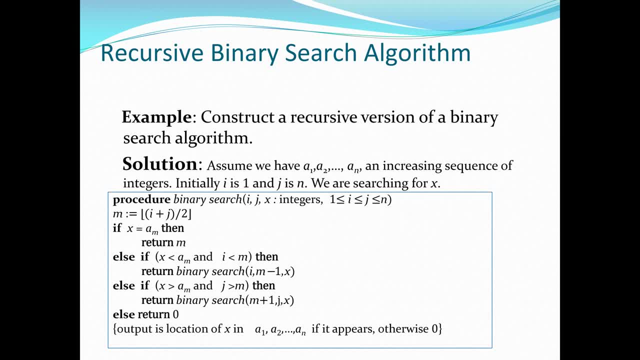 If it's lesser, we'll go to greater. Then we'll repeat the same item with the same step. again The new list, half of the new list. we find the middle. Then we compare again. If it's greater, then we find the middle. 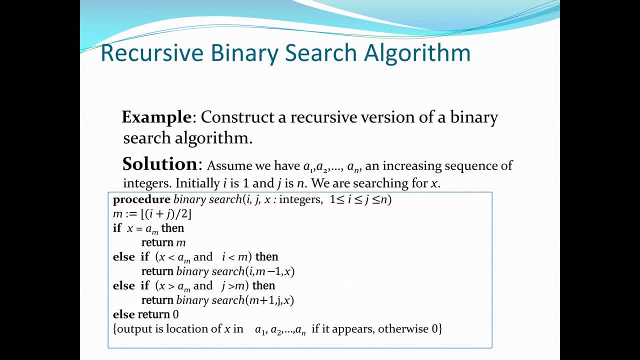 If we forget about the lesser set, then we'll find middle again. So you can see that that's why it's called binary search. Always we divide the list into two. One part of the list we are not going to search, So this will save a lot of time. 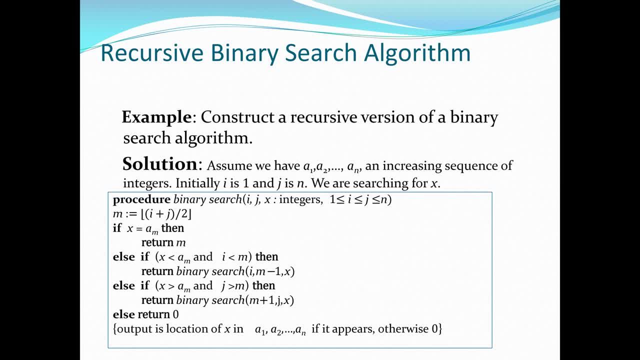 We don't need to do all the comparisons. So that's the whole concept here. Now we can use this. We can write this algorithm using loops- interactive- But we can also design it using recursion or recursive, And that's what we're going to do. 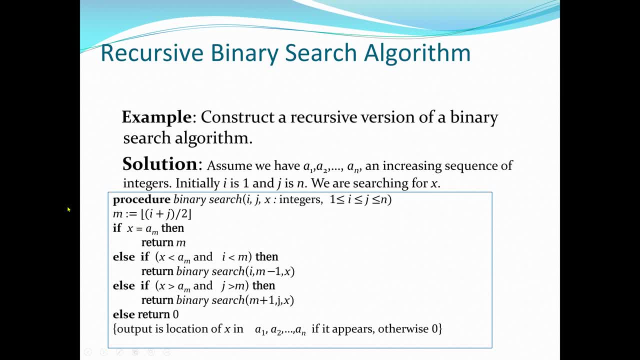 We are doing here. So we can see that the first thing we do is the m is the middle value. So this i and j is like our index. Here we are assuming we are using a ray, So i and j can be our index positions. 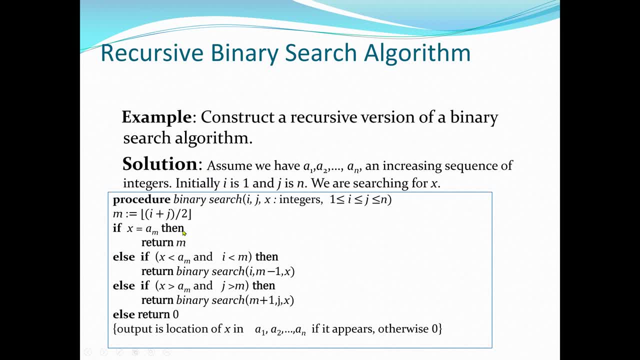 So i plus j, divided by 2, will give me the middle value, Again the index position, the middle. Now I'll say that, okay, if a m or f f is equal to a m, then we'll return m. 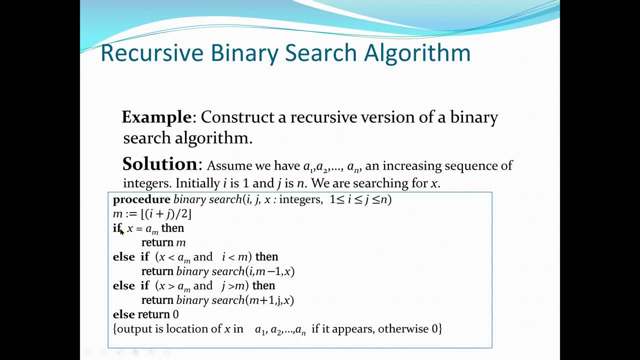 This means we have found a search key. The search key is the same as the middle value, a, m. So in this case, we return the m, because our goal is not to return the search item. We know the search item. We just want to return the position, which is the index in terms of array. 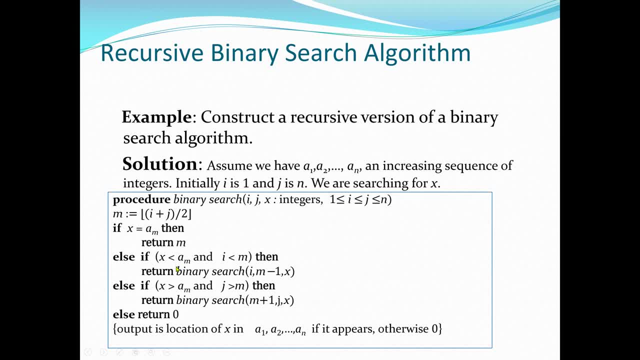 Else it's okay. if the search key, let's say the search key a, m is greater than x, Then we go to the greater section, So we go to, and also the middle is greater than the i, Then of course we are going to the i and m minus 1.. 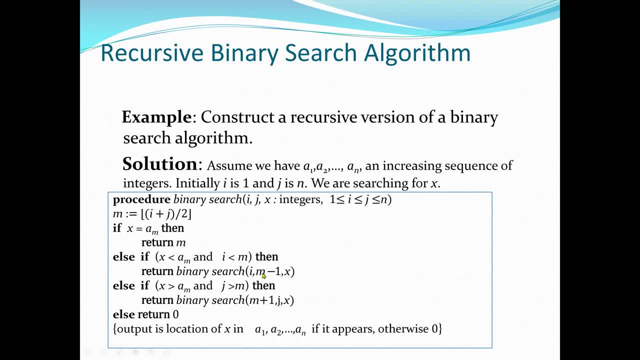 So, which means we are going to search at a greater side, Because here we can see that a m Is greater than s, or s is less than a m, and also i is less than a m. Otherwise, the other way, if s is greater than a m. 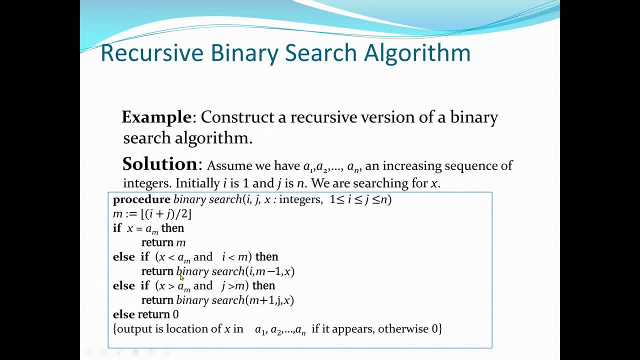 which means we're going to the lower side because a m is low, So in this case it will take us to the lower side. So those are the. that's the now. this is our recursion. is what is happening here? This is our recursion. 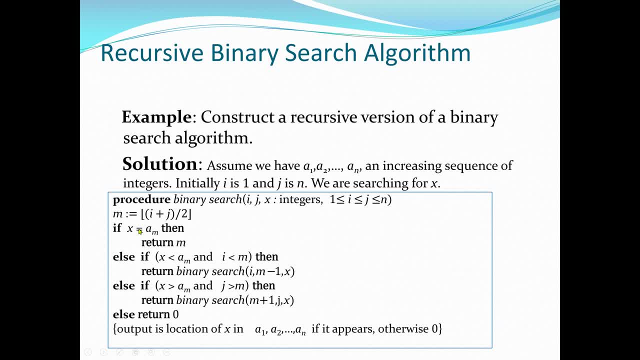 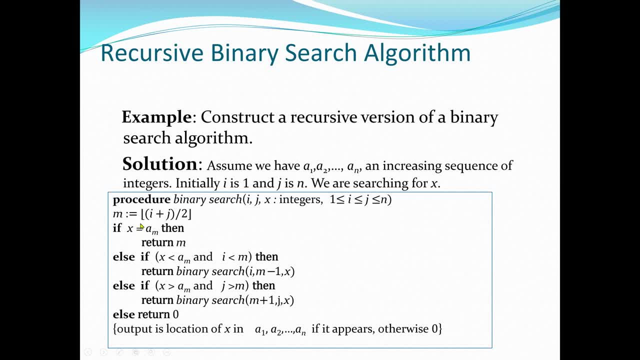 When the search key is the same as the middle value, you stop. Otherwise, if the search key is less than middle value. So this means middle value is greater than the search key. Then we go to the lesser side of the item. Now, if the middle value is great is lesser than the search key. 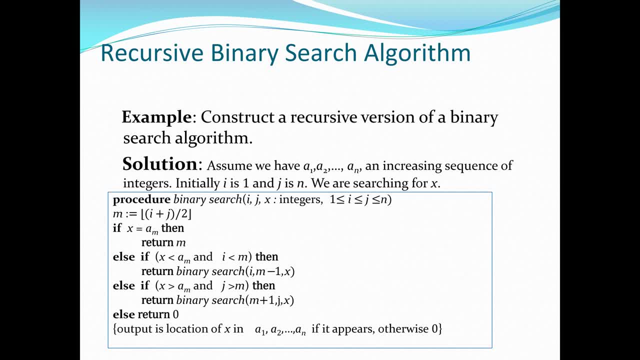 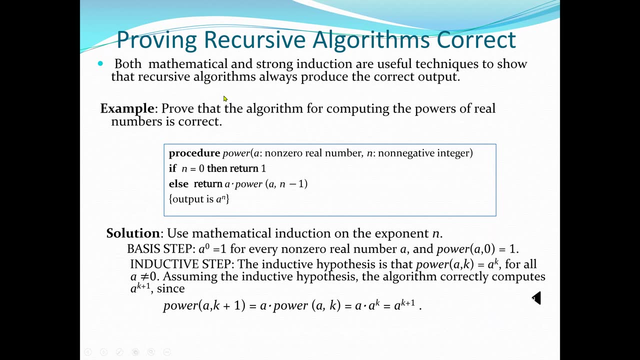 That search key is greater than the middle value. Then we go to the larger area from the middle And these are recursive because we can see the function is calling itself. So they say we should prove the recursive for guardian if it's correct. So both mathematical and strong induction are useful techniques to show that. 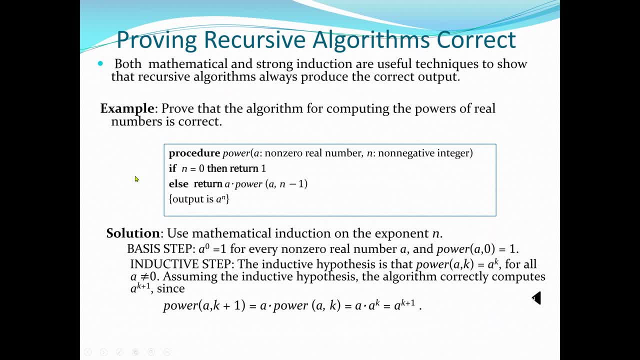 recursion is correct And we can see for guaranteeing always produce the correct result. So for example, if they say we should prove that they're already for computing the powers of real numbers is correct. Here we have the function in power. It takes couple of arguments: a non-zero real number and n non-negative number. 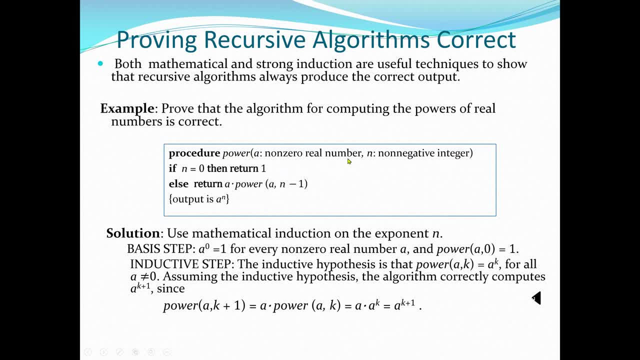 because this is power. a is like our base and n is our exponent. So we say that if n equal to zero, which means If the exponent is zero, any value raised to the power of zero is one. So we return one. That's our base case. 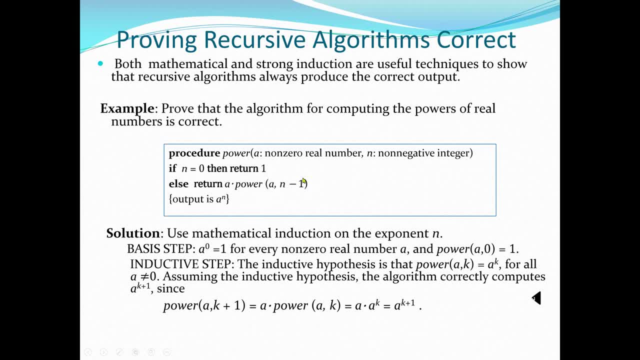 As we return a times power, a n minus one, which means if I take one value from the, let's say I have three cube. If I write three times three, square is the same. So that's why we have n minus one in this case, to the power three minus one. 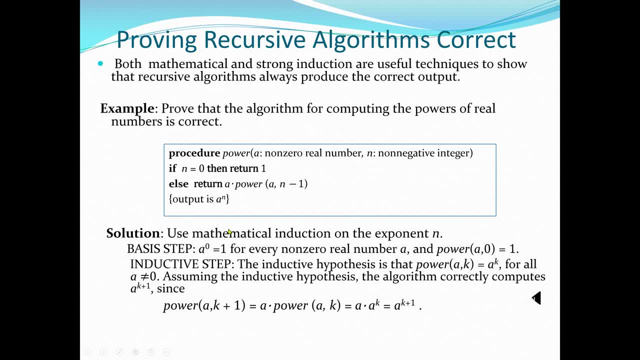 If I take one three out. Now, this is our solution. Now we want to prove it is correct. So what we do? we use the mathematical induction on the exponent n, because n is our input, So we have to use most of the time again, always we use proving. 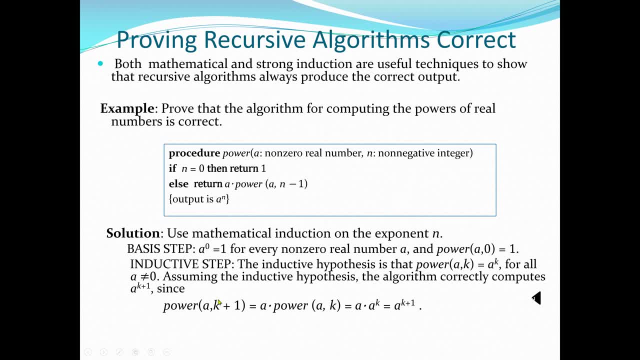 We always use the input, So the input is n and n happy to be the exponent, Because power a to the power n. So in this case the basis step will be what a to the power? zero is one The lowest you need for n would be zero. 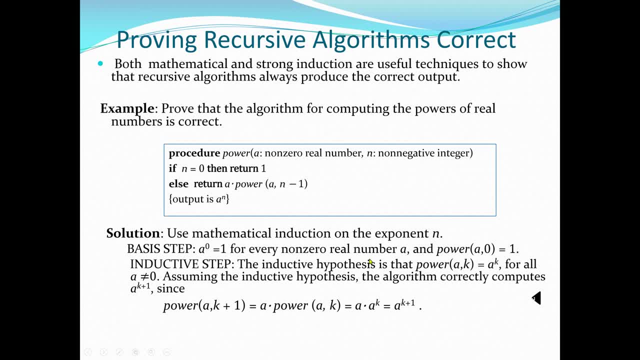 And the is one for every non zero real numbers, a. the base is A. the base would be a positive value and not zero. And the power A and zero, which means a to the power zero, is one. So that's our basis. step, the lowest unit. 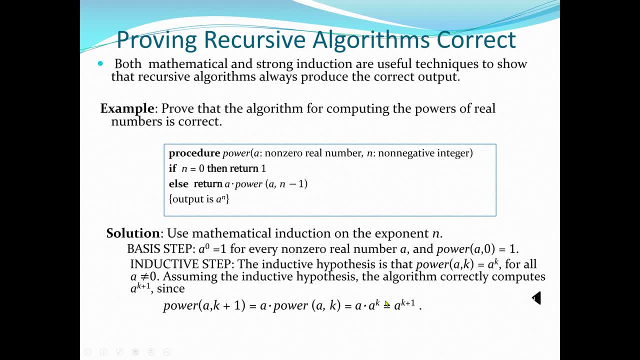 Now the inductive step, that we say the inductive hypothesis is that the power akarnya is equal to a, to the power k for all a, not equal to a to zero. Now we are assuming the inductive hypothesis, the algorithm correctly compute. 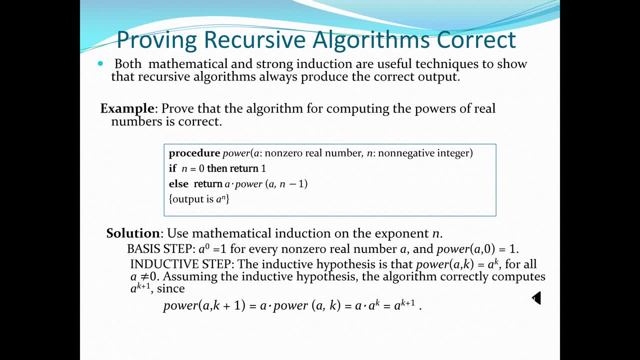 a k plus one. Now, since power a and k plus one equal to a times power a and k, because we plus one, we take one a out. We use the a multiplied by power a k. So this is the same as saying a times a k, which will give us a k plus one. So here we have proved that. 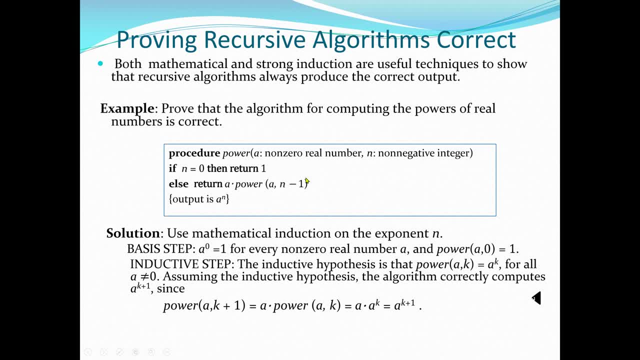 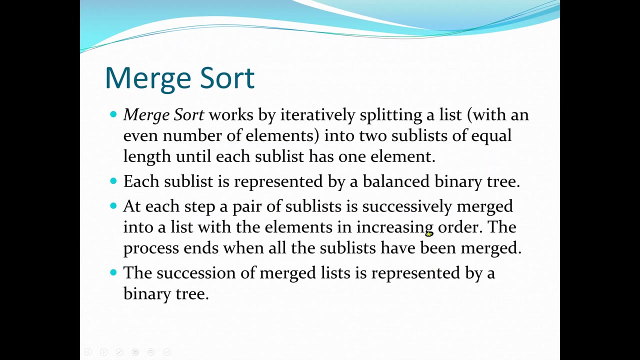 again, this recursive algorithm is correct Because we move from a to a plus if the k is the exponent. So we get a times a to the power. k is the same as saying a k plus one. So next we go through the merge sort. Merge sort works by again interactively splitting. 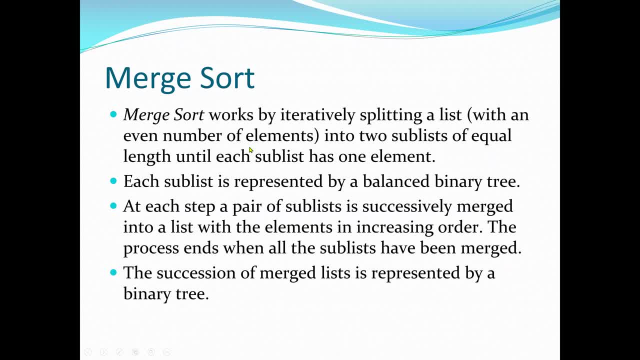 a list with an even number of elements into two siblings of equal length, until each sub list. each sub list has one element. So what we mean is actually- we will see a diagram in the next slide so we may go through that- But what we mean by merge sort is that we 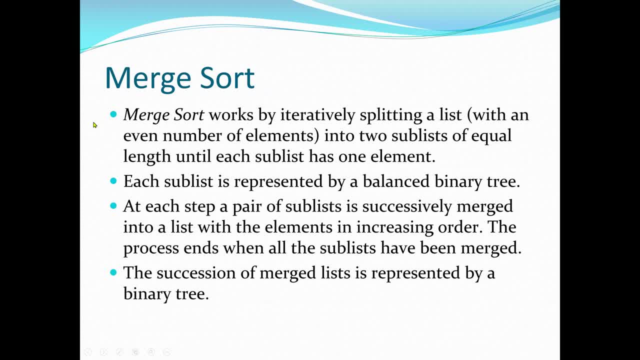 have a list of items. We want to break it step by step until we have only one unit. Then we merge them together and putting them in correct order So we may have. each sub list is represented by a balanced binary tree And at each step a pair of sub lists is successfully. 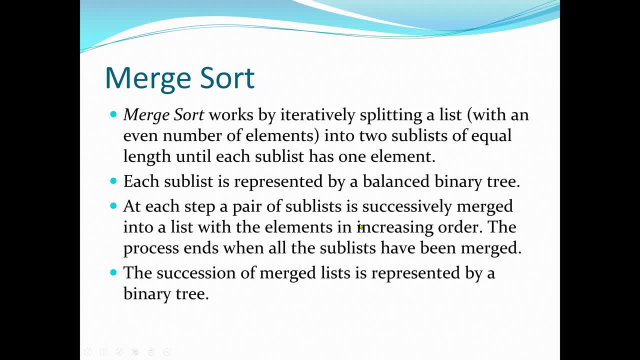 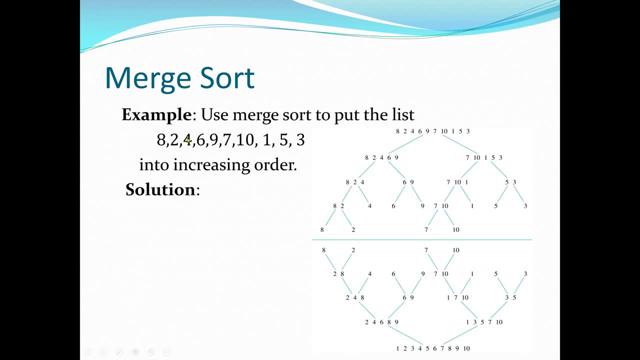 merged into a list with the element in increasing order. If your sorting is in ascending order, increasing order. Otherwise we can also be decreasing order. So this is a very good example. We want to sort 8,, 2,, 4,, 6,, 9,, 7,, 10,, 1,, 5,, 3.. There are 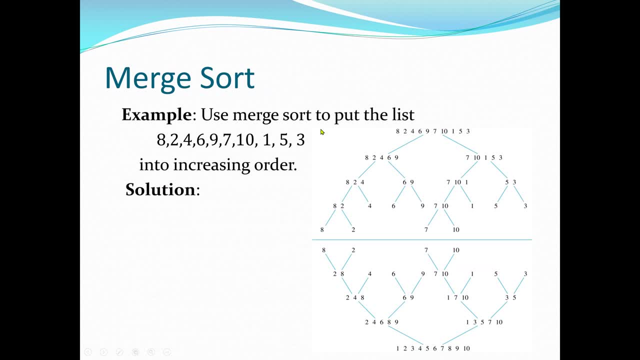 so many sorting algorithms in computer science. Example can be from bubble sorting we saw selection sorting. There are so many of them, But here we are using merge sorting, So we can see that each one use different algorithm. But the goal of sorting is that we want to. 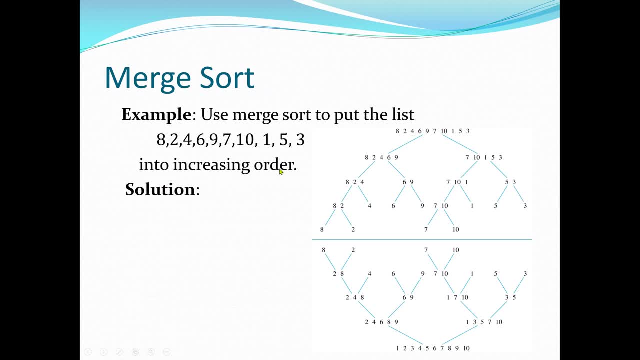 optimize our problem. So we need a sorting algorithm that do less comparison, which means it's more faster. So you can see that this is the list of the item in the diagram we are sorting. What do we do? We divide the sub list into two, One to the left, 8,, 2,. 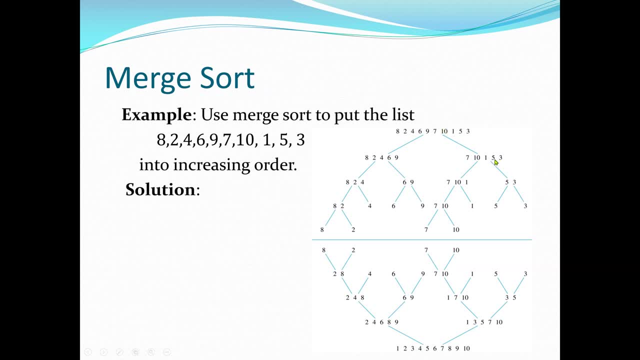 4,, 6,, 9.. The other to the right, 7,, 10,, 1,, 5,, 3.. Then we do the same thing again. We divide the list into two sub lists again. So we have three values here: 2. Then we divide. 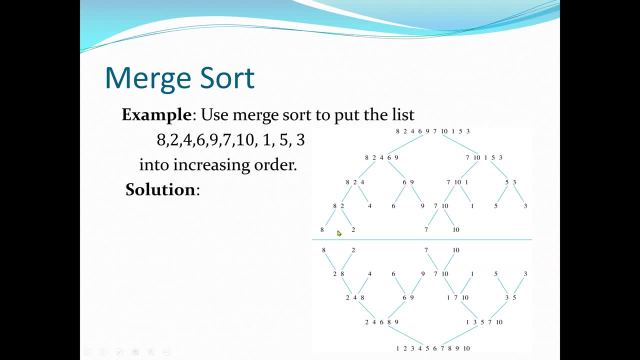 it again: 2 and 1.. Then the two we divide again. We are going to again divide the items until we have each individual item. So here we can see each individual item: 8,, 2,, 4,, 6,, 9,, 7,, 10,, 1,, 5,, 3.. Okay, Now we have to read: This is where we will do our merging. 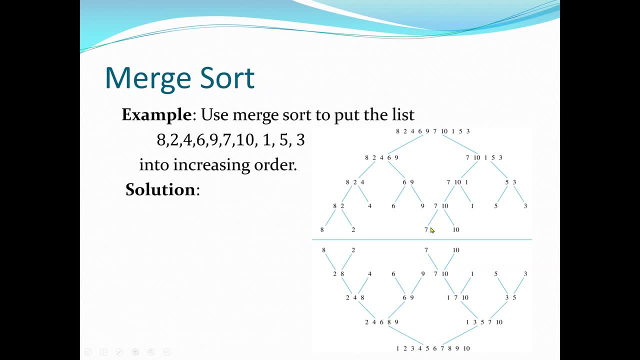 We start the merging from the down. So first I have 8, 2.. In the correct order it will be 2, 8. So we merge it to 2, 8.. 4 is by itself, I will leave it. 6 is by itself, I will leave. 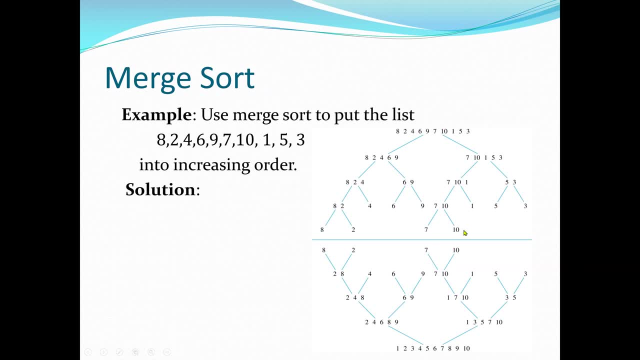 it here 9 also. I will leave it. But here we have 7, 10. So when we merge it, we still get 7, 10.. And here we have only 1,, 5, and 3.. Now we read this section. now This section. 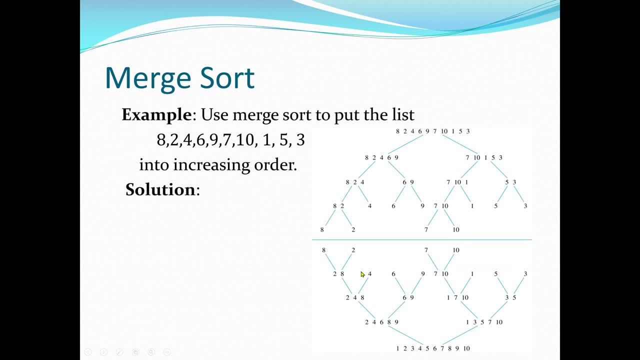 means we have 2,, 8,, 3.. And here we have 1,, 5, and 3.. Now we read this section. now This section means we have 2,, 8, and 4.. So we have to put it in order, So it will be 2,. 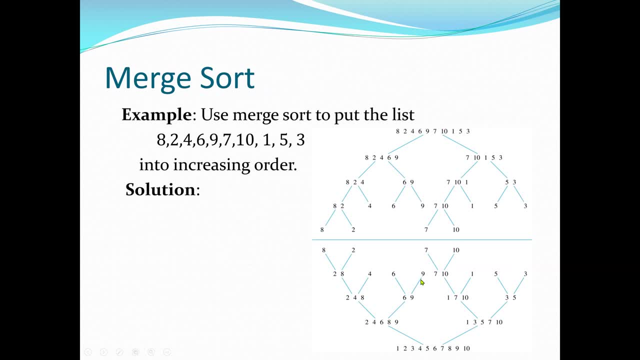 4, 8.. So we have 2,, 4,, 8.. Here now we have 6, 9.. So when we put it in order, we have 6, 9.. And 7, 10 will be 7, 10 down, And then 5, 3 will be 3,, 5, 10, 1 will be 1.. Here we 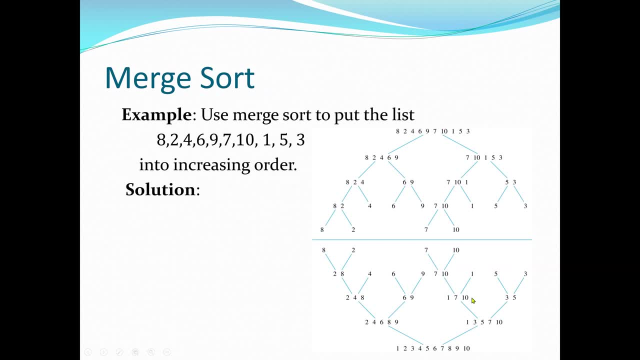 have the 7 also, So it will be 1, 7, 10.. Now, if I want to reach this section, I have 2, 6, 9.. 2, 5.. So I have 2, 4, 8, 6, 9.. So I will put them in order. So I will get 2,. 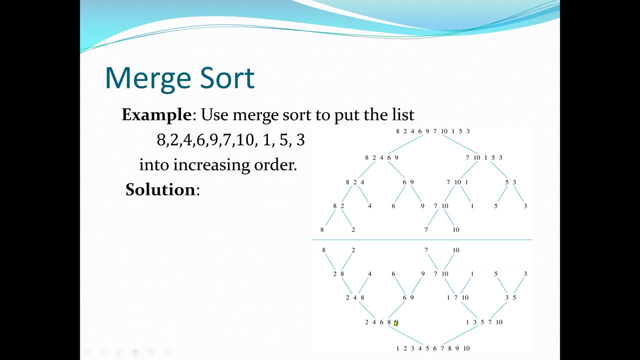 4,, 6,, 8,, 9.. And that is 2,, 4,, 6,, 8,, 9.. That is almost all these. Then here we have 1,, 7,, 10.. And also we have 3, 5.. 1,, 7, 10.. 3, 5 to merge. So we 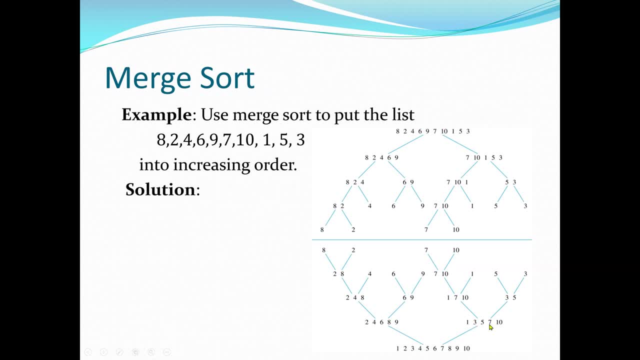 get 1,, 3,, 5,, 7,, 10.. So now we have the last part. now We have only 2,, 6,, 10.. Oh, 3, 5. 9.. Yeah, Only 8,, 7, 10,, 1, 9.. 6,, 7,, 10.. Punder, End of session Regressed And 3, 6, 10.. 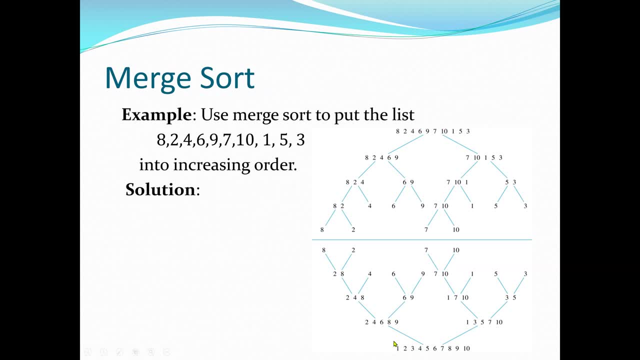 only two sub lists. now we have to sort them and put them in order. so we get one, two, three, four, five, six, seven, eight, nine and ten, and that's what we have here. so merge salt, the first algorithm, first step: you want to break your item into one unit, then later you merge them by. 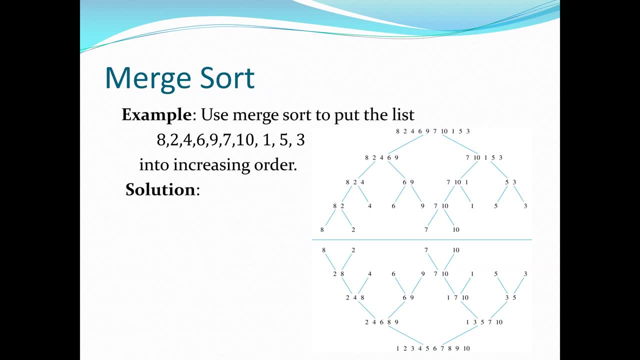 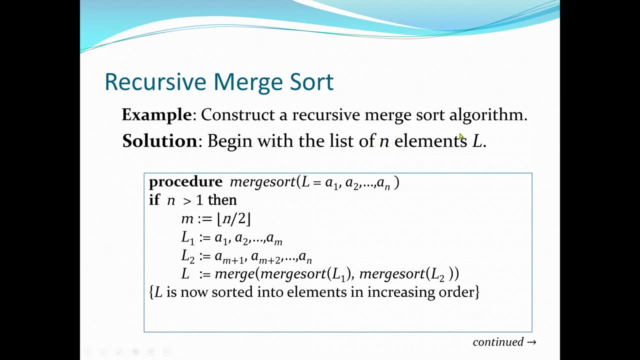 putting them in the right positions. so in the recursive method we say here: construct a recursive match sort algorithm. solution is: we begin with a list of n elements, l. so let's sort l equal to a, y, 2 up to a n. now we say that if n is greater than one then we divide the item into two. 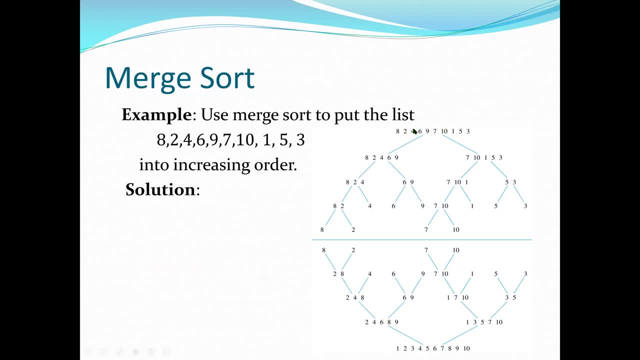 you remember the diagram here we have. if the item is greater than one- which means we have at least few items here, let's say two or more- we need to divide into two. always we divide the atoms into two when we are merging, then we combine two at a time. so that's why, here again, we say: 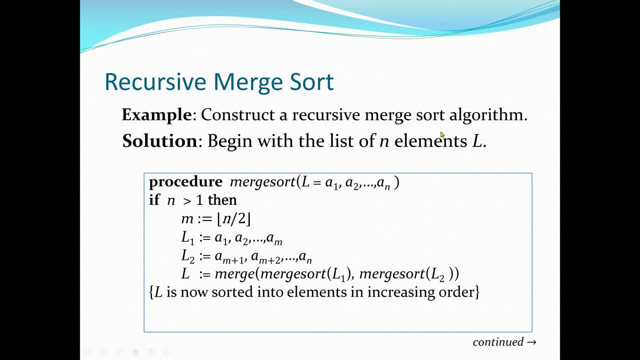 construct a recursive image, sort of bar again. so we begin with the list of n elements. so again the recursive mesh sort. uh, here again the social construct, the recursive mesh sort. begin with the list of n elements. so these are the elements: a1, a2, up to a n. so first we said okay if n is greater than one. 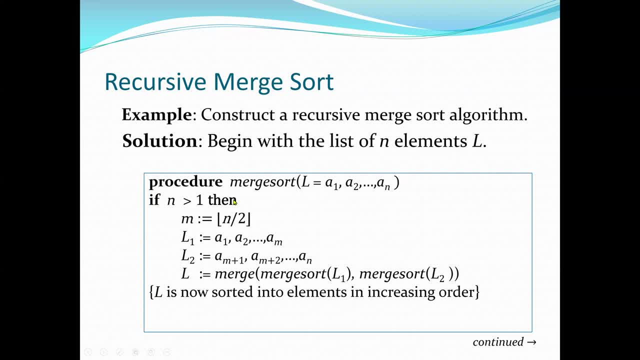 we have a lot of and we have items. so we find the main, main elements of the list of elements. so we need m. m will be: we divide the list into two. we divide the list into two to m. then we list l1, as we saw in the diagram. then we have, let's say, the left and right, l1, l2, the items. 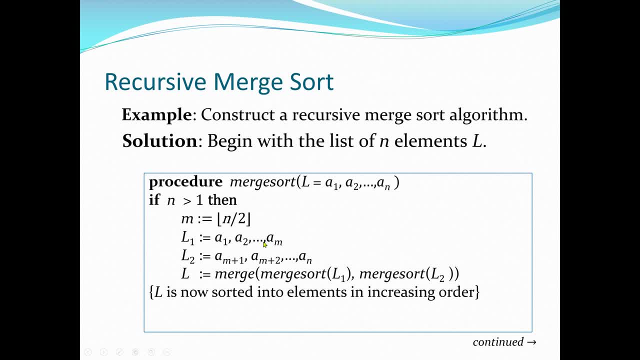 so first, to the left to be a1 to am, to the right to be m, a, m plus one to am, which is the total. then we are going to call the function merge um to merge the left and the right together through sorting. but here we say l is now sorted into element in increasing order. 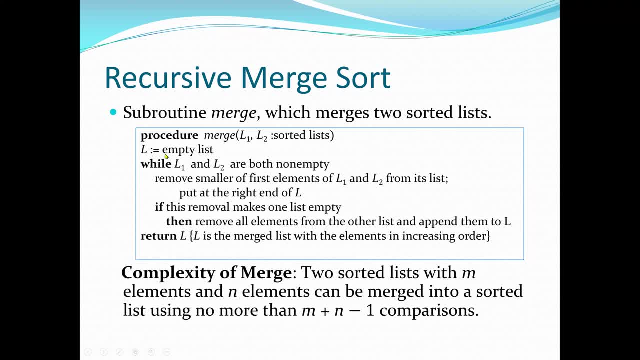 so this is the algorithm now. first, l is empty ls, while l1 and l2 are both non-empty, which means we have an item. ln 2, are both nonempty, which means we have an item. we should remove the smaller or the first element. 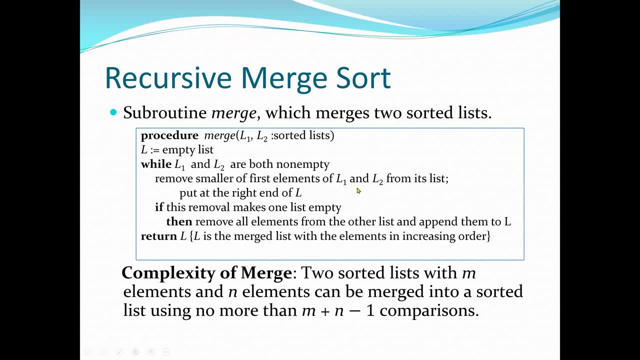 we should remove the smaller or the first element element of L1 and L2 from its list. then we'll put at the right end of L. Now, if this remover makes one list empty, then we'll remove all the elements from the other list and append. 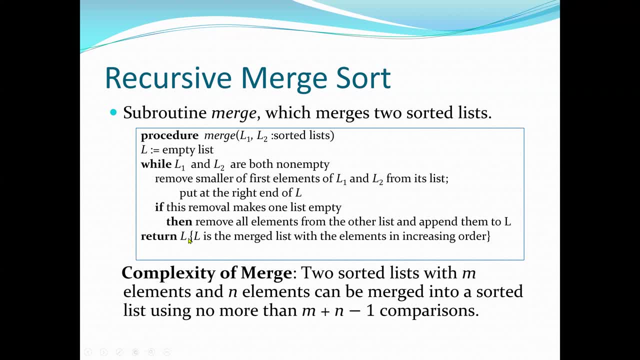 them to L, Then we'll return L, So L will be our merge list with elements in increasing order. Now the complexity of the merge sorting algorithm is that we have two sorted lists with M element and N element, And this can be merged into a sorted list using no more than M plus N. 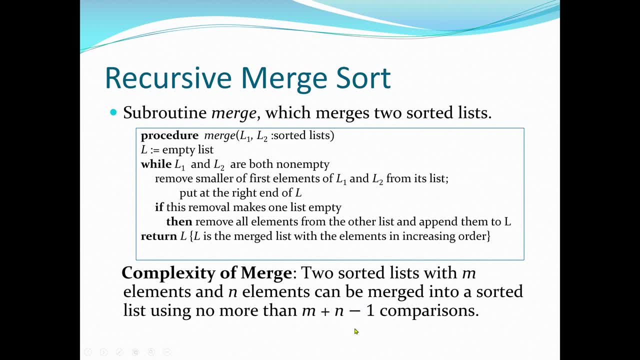 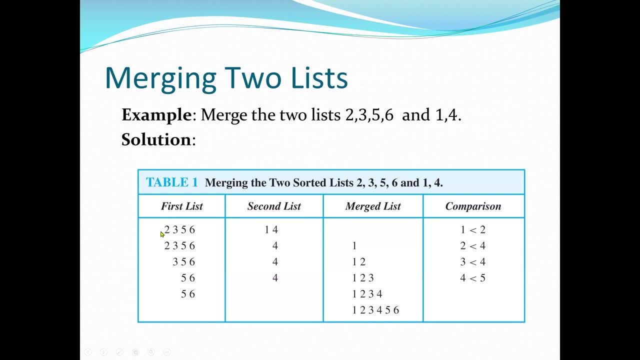 minus 1 comparisons. So example given here: we want to sort the item 2,, 3,, 5, 6, 1, 4.. So that's our first list. our second list. So first list, we can see that 2,, 3,, 5, 6, 1, 4 is sorted. So the comparison 1 is less. 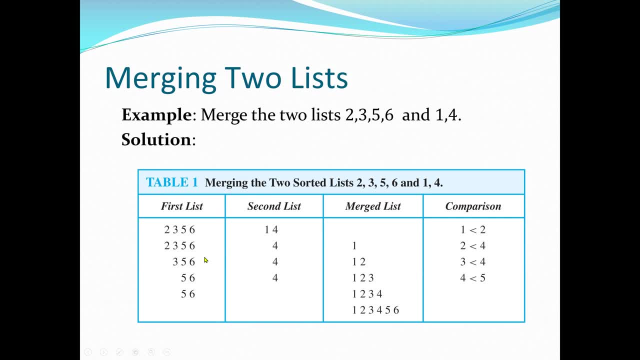 than 2.. So next we have 2,, 3,, 5,, 6.. We merge one out, Then next we have 2,, 3,, 5, 6,, 1, 4.. 3,, 5, 6, because we take 2 out, Then next we need 3 out, Then next we need the 4.. So 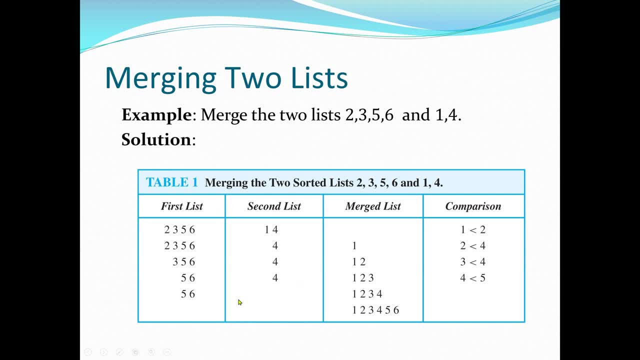 after we take the 4 out, we don't have anything in the second list. Then we'll bring the 5 and 6 together. So this is again after we break the element into smaller unit: individual 1, 1.. The process: 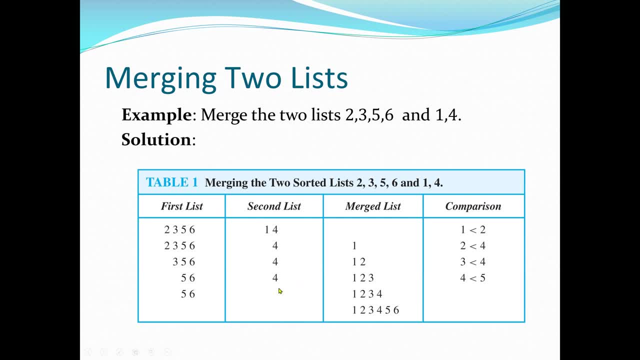 of merging the two sorted lists is what we just did now. So I have two sorted lists. I'll look for the lowest For both two lists. the lowest is 1,, the next lowest 2,, 3, and then we keep going up to the end. 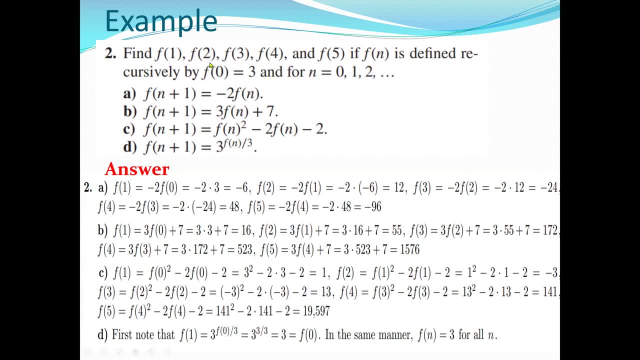 So let's see some examples here. Here they say we should find f at 1, f at 2, f at 3, f at 4, f at 5.. If f at n is defined recursively by f at 0, equal to 3, and f at 4, n, equal to. 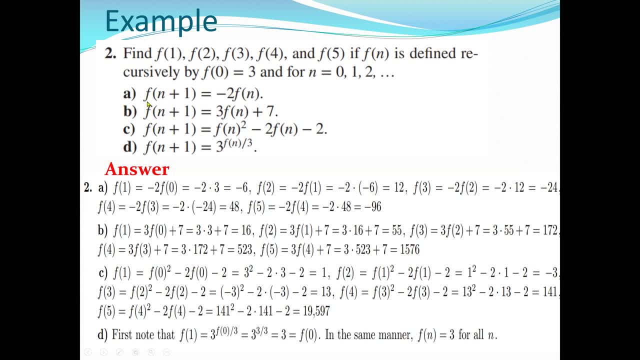 0, 1, 2.. So first we need to find f? n plus 1.. And here they say it's negative: 2 f n. So this means if I'm looking for f at 1, it will be negative, 2 f at 0,, which will give. 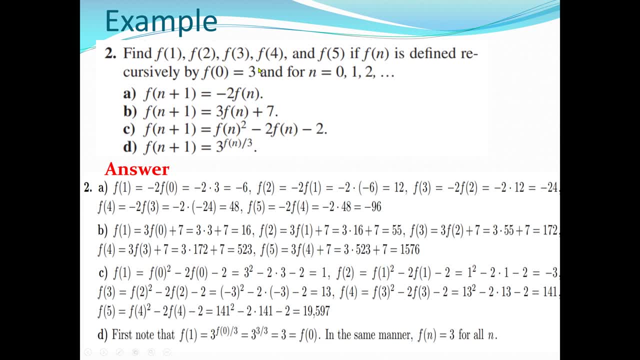 me negative 2 times 3 because again f at 0 is 3.. Now if I'm looking for f at 2, I'm using the a- again Negative. 2 f at 1, because previously f n plus 1 minus 2 f n. So it will be negative 2 times negative, 6.. F3: the same thing, negative. 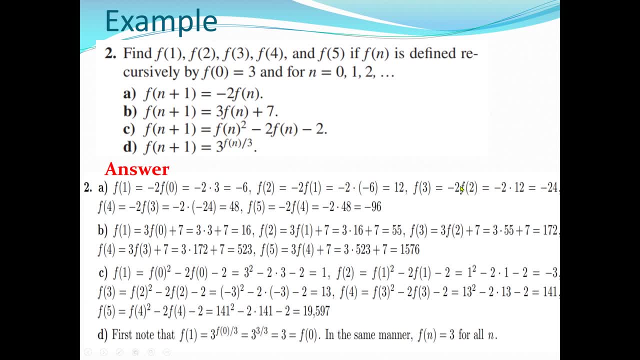 2 times f at 2.. We have this. Okay, We have the answer. Then f at 4 will be negative 2 times f at 3.. Then f at 5 will be negative: 2 f 4.. So we can see n plus 1, the previous n we are using. Then times 3 plus 7.. The same. 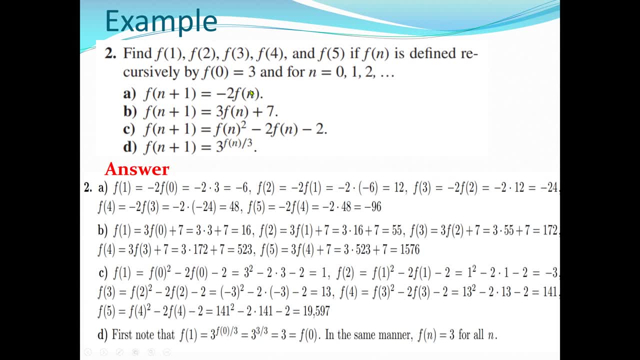 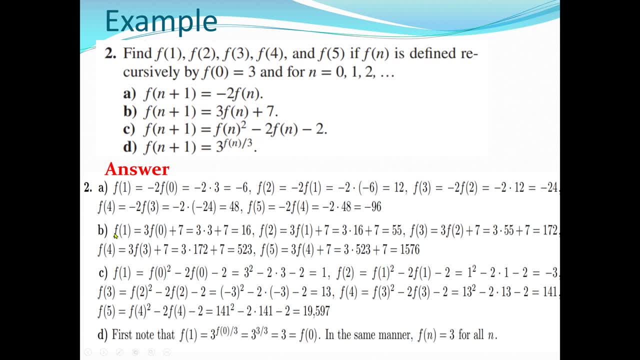 will be 3 times the function plus 7.. So in b we know f at 1 will be the previous, here will be the previous f at 1 and f at 0 plus 3.. So 2 times f at 0 plus 3, which will be. 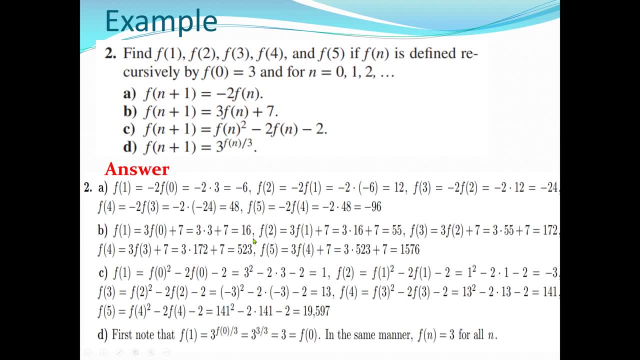 3 times 3 plus 7 system. Now f at 2 should be f at 1 times 3 plus 7. So f at 1 times 3.. The function is f n 3 plus 7. We know f at 1, we just find the result. The result is 16.. So we say 16 times 3 plus. 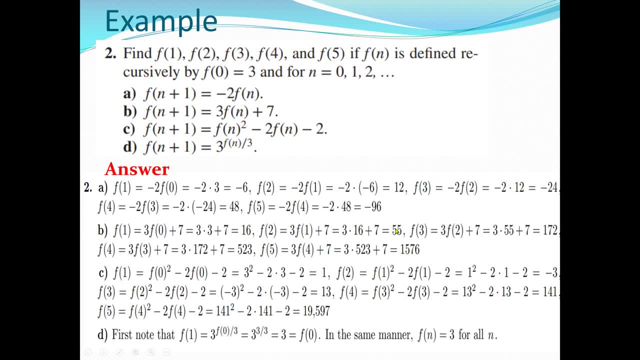 7.. Then let's do one more: f at 3, b 3 means we have 2.. So it will be 3 times f at 2.. f at 2, we just find the answer right now. So we plug in the answer, which is f at 2 plus. 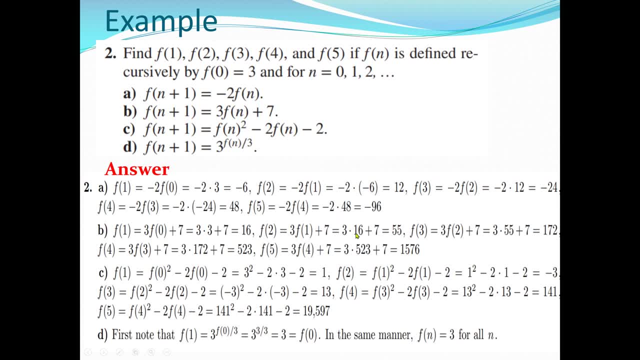 7. Then we plug in the answer, which is 55. Then plus 7.. The same thing applies to the b, c, d. Let's say, if we use c, C, we have f? n plus 1 f n. 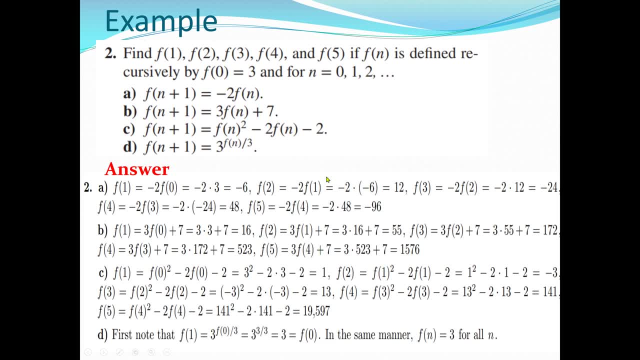 square minus f, n minus 2.. So this means if I'm looking for f at 1, I need f at 0 square here, which will be 3 square. So let's go b, So we get 3 times 3.. 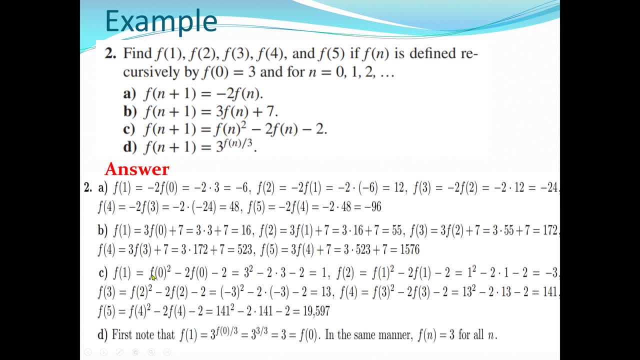 No, actually we are doing c, Sorry c. So we see that we get f at 0 all square minus 2, f at 0, again minus 2.. So that will give me 3 square minus 2 times 3, then minus 2, which will give me 1.. Now 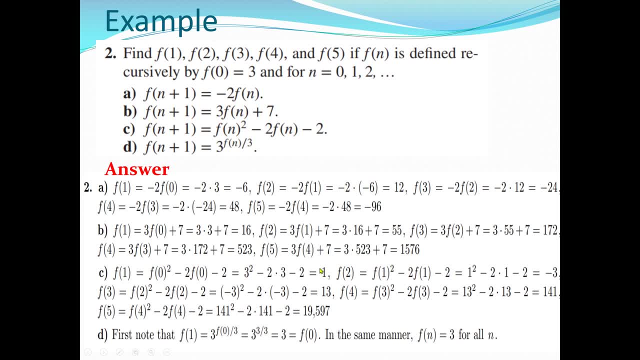 f at 2 will give me f at 1 square, which is f at 1 square, And f at 1 equals 1.. So we F at 1 is 1, so we get 1 squared minus 2 times F at 1, which is 1.. 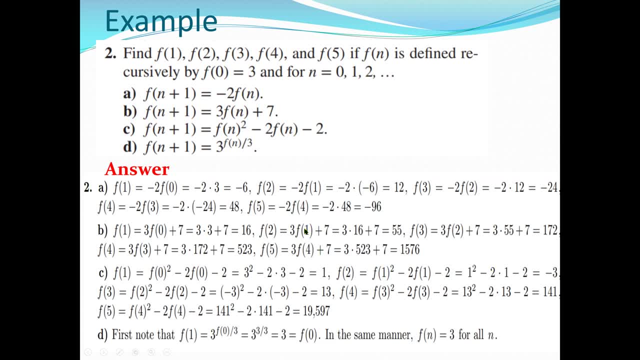 Then again we do the calculations. So again let's do only one for D: F at n plus 1,, 3 to the power F at n divided by 3.. So if I'm looking for F at n plus 1,, 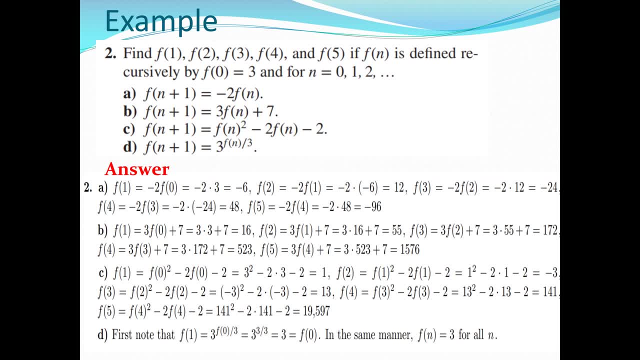 it means, if I'm looking for F at 1, then it will be 3 to the power, F at 0 divided by 3.. So let's see the D here: F at 1 will be 3, F at 0 divided by 3.. 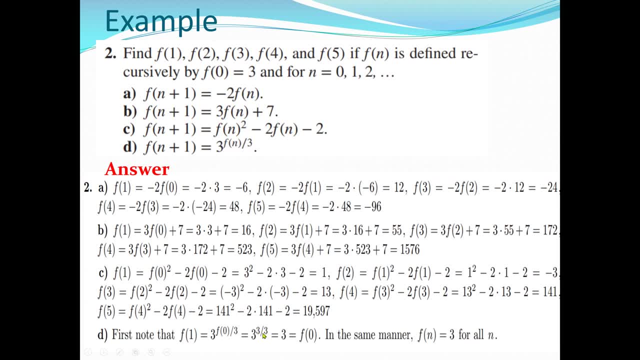 So this will give me 3 to the power 3 divided by 3.. And my answer will be 3.. The same thing for 1.. Since now I know F at 1, F at 1 is 3.. So I'll say 3 to the power 3 divided by 3.. 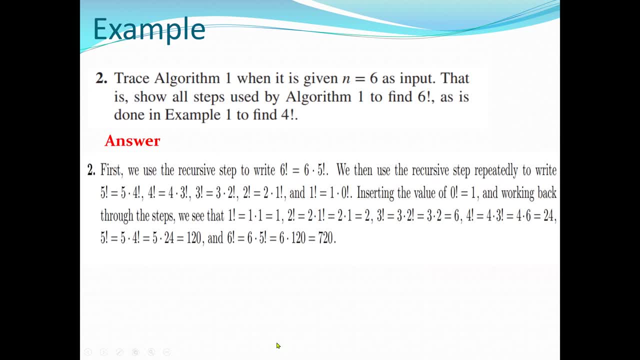 So let's see the D here. So next is tracing algorithm 1. when it's given n equal to 6 as input, The algorithm 1 is finding the factorial of a number. So here we need to show the step used by algorithm 1 to find 6 factorial. 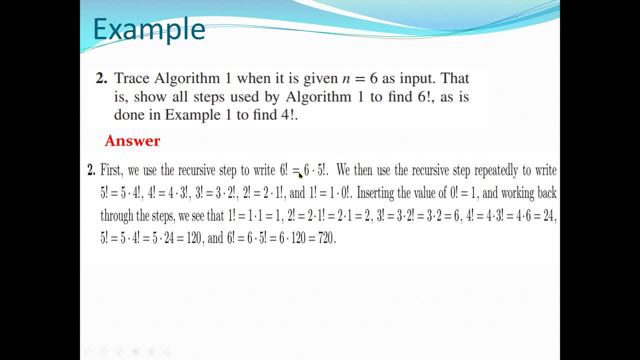 So first, we know that 6 factorial is the same as 6 times 5 factorial. We know that 6 factorial is the same as 6 times 5 factorial, Which means we get cn times the function n minus 1, which is 6 times 5 factorial. 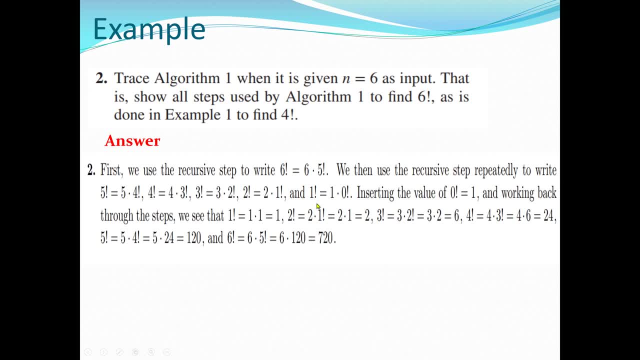 Factorial is the function, so we have to see the function n minus 1.. Then we can use the same recursive step repeatedly to write 5 factorial, which will be 5 times 4 factorial. 4 factorial will be 4 times 3 factorial. 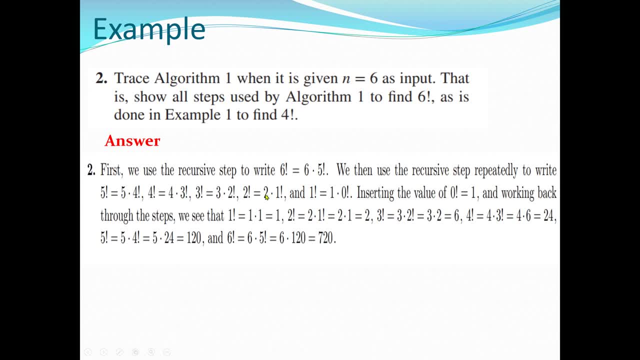 3 factorial will be 3 times 2 factorial, Then 2 factorial will be 2 times 1 factorial. And the last 1 factorial is 1 times 0 factorial. 0 factorial is 1.. And walking back through the step we see that 1 factorial is 1 times 1,. 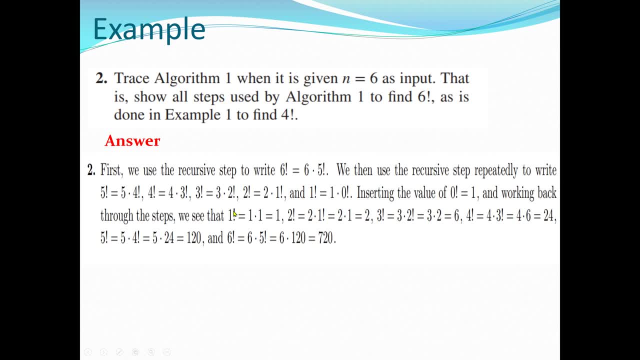 equal to 1.. Then 2 factorial is 2 times 1 factorial, which gives us 2 times 1.. Then 2 and 3 factorial will give me 3 times 2 factorial, etc. So we keep doing it until we reach 6.. So 4 times 6 is 24.. 5 factorial will be 5. 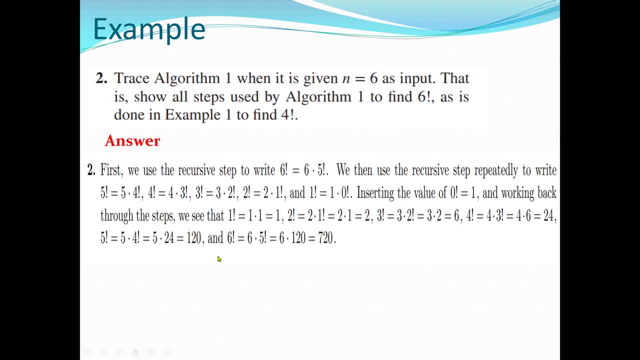 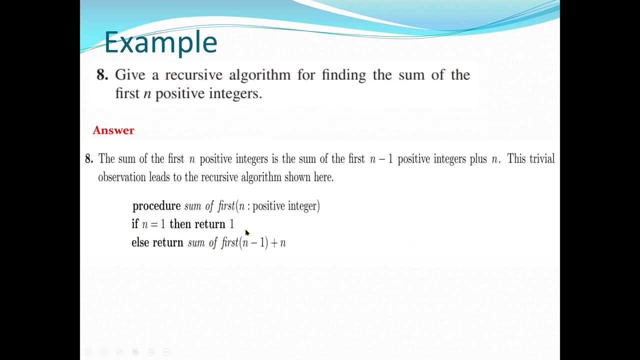 times 4 factorial, So it will be 120. Then 6 factorial will be 6 times 5 factorial. 6 times 120 will give me 720. So the final result will be 720.. So next example says we should give a recursive algorithm for finding the sum of first n positive. 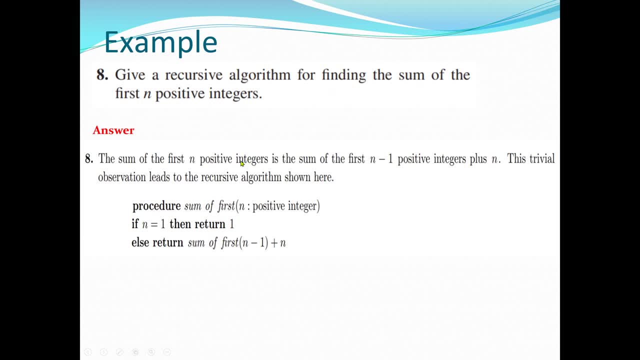 integers. So here we can say: the sum of the first n positive integers is the sum of the first n minus 1 positive integers plus n. OK, So we write the function into the sum of firsts. So we are starting the n and also.